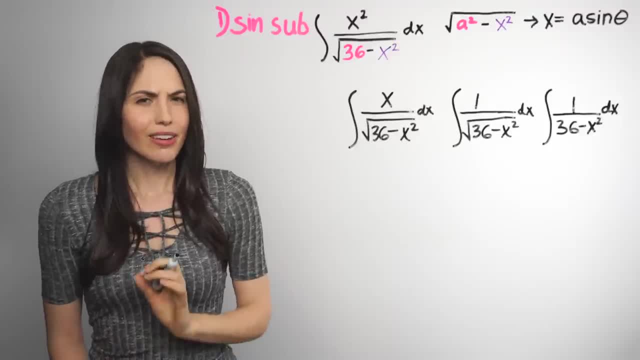 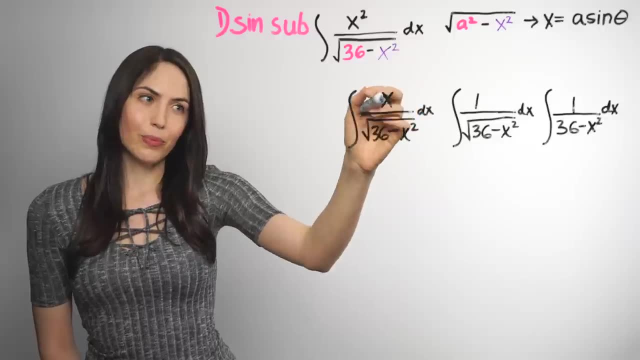 something like an inverse trig integration rule. Very smart. You should check to see if you can Like. if we had had instead just x on top, we could have done u substitution and the power rule, but we don't. We have this x squared. 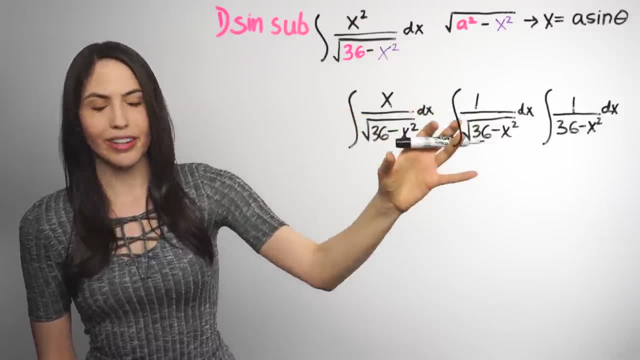 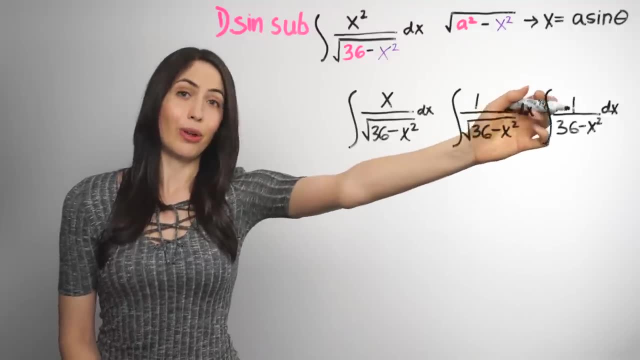 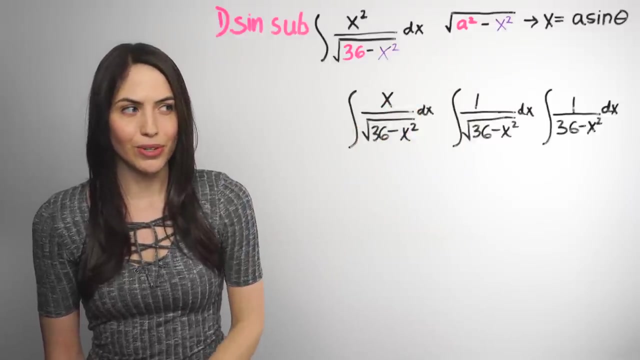 If we had just a 1 on top, it would have fit perfectly. the inverse sine integration rule. That would have been nice, but we don't have that. Or like this: 1 over 36 minus x squared, That is something called the inverse hyperbolic integration rules. So that would have been an. 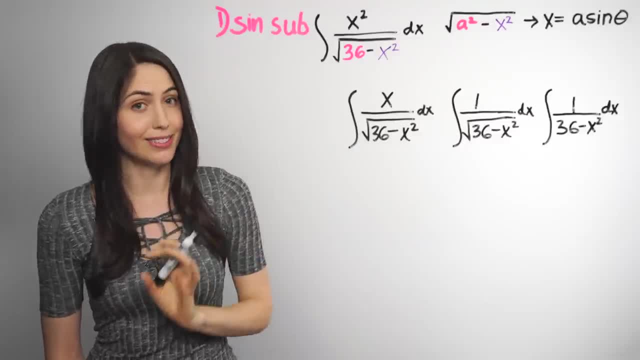 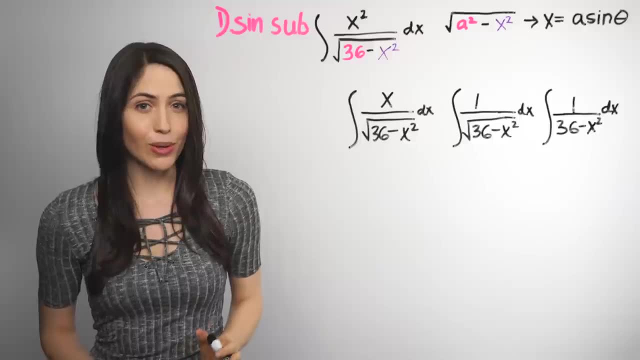 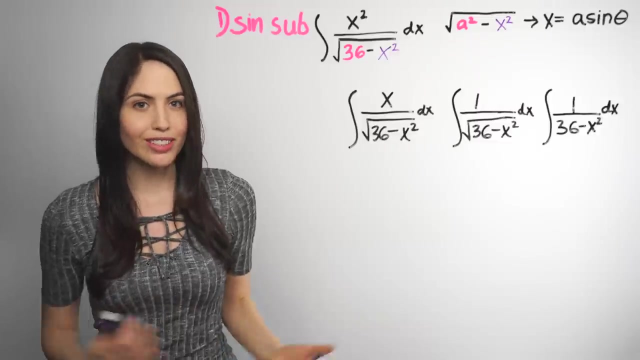 inverse hyperbolic cotangent or tangent- Yeah, those exist. We don't have that. We can't use those. You should check first. if you can't use those and you can't use something from the table of integrals or integration by parts or partial fractions or any other technique, what can you do? 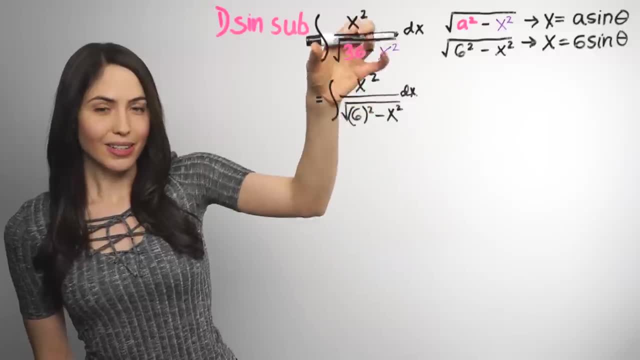 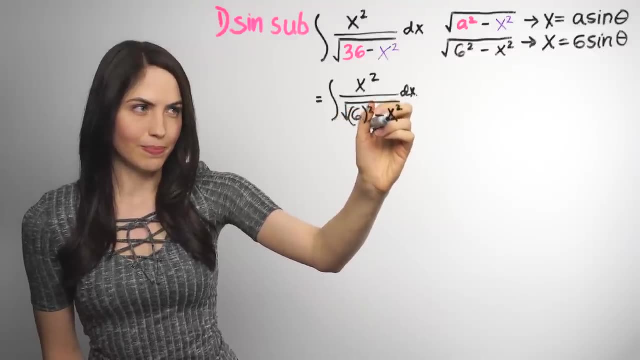 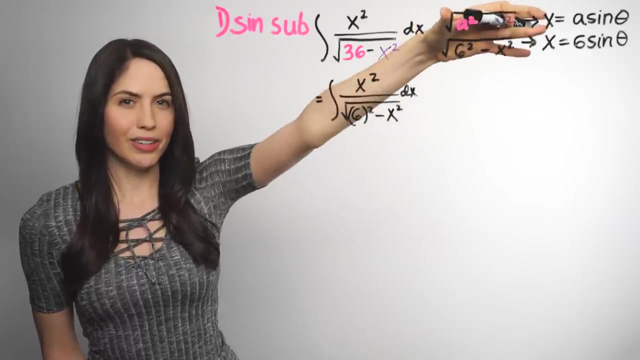 We can do a sine substitution. So if you take what's under the radical and rewrite it as a number squared minus x squared, or here a number squared minus x squared under the roots, and compare it to the formula for sine substitutions, you'll see that a is 6 for us. 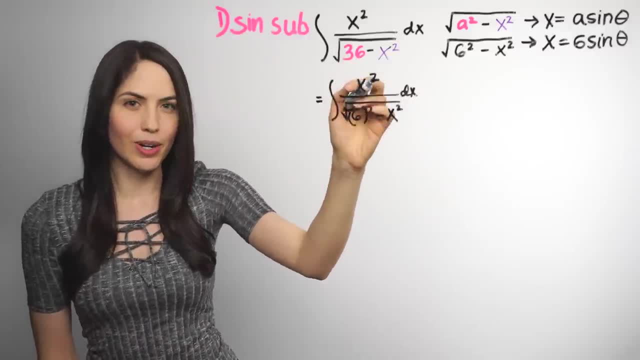 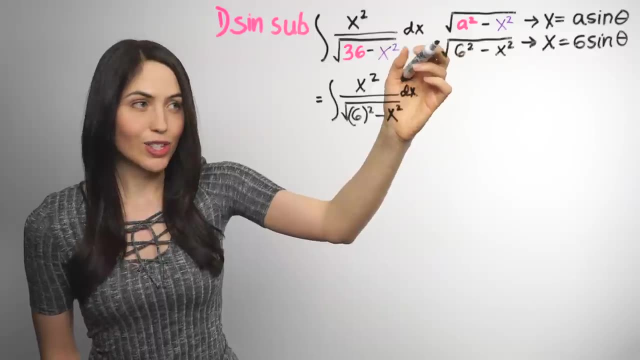 And, by the way, if you ever saw a 1 here like 1 minus x squared, 1 is 1 squared, so a would be 1 in that case, But our a is 6, so our substitution is going to be: 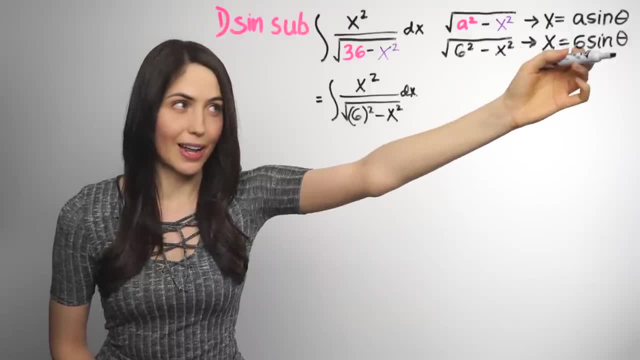 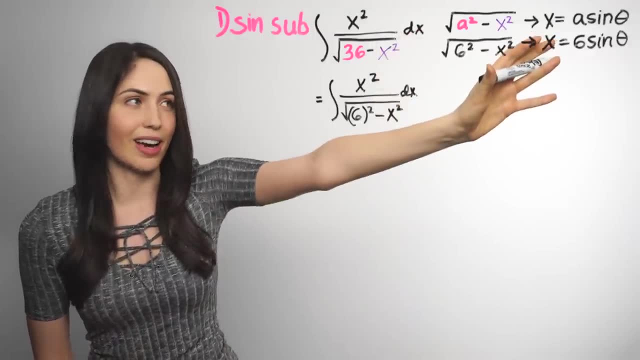 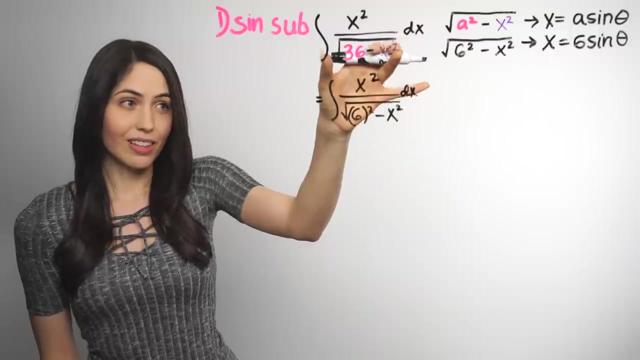 x equals 6 sine theta. That's our substitution. Not that you would know that right off the bat. I mean, I know this is coming out of nowhere right now, But you'll see how it helps in a second. The next step is to take the radical out on its own. 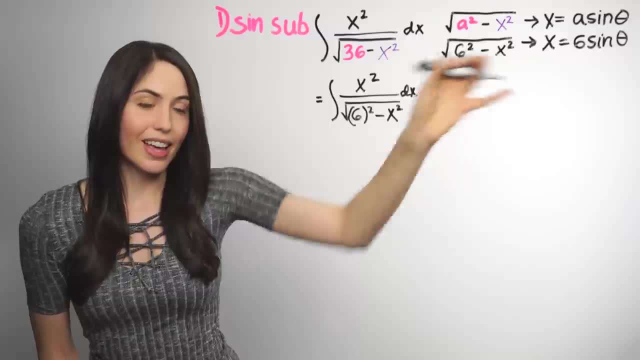 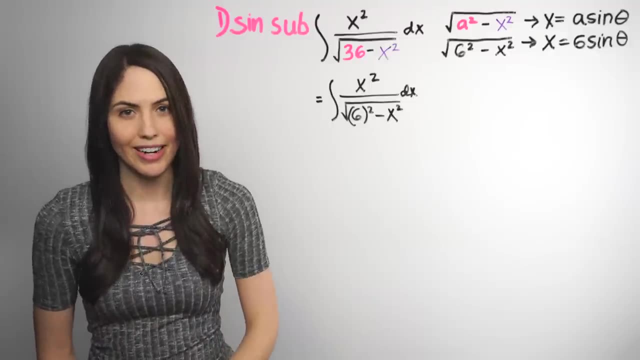 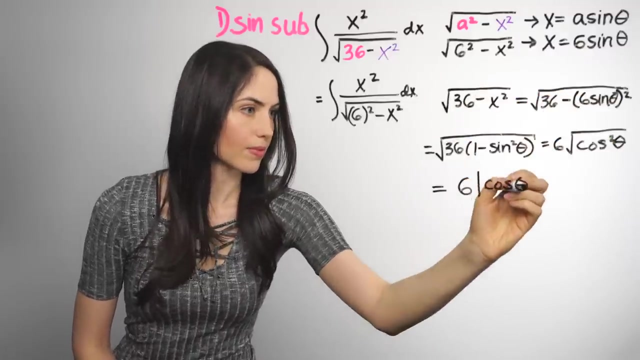 and plug in this for x and then see how it simplifies, because it's going to break down the radical and simplify the roots through the wonder of Pythagorean identities. So So let's try that. So we take the radical and plug in our substitution. 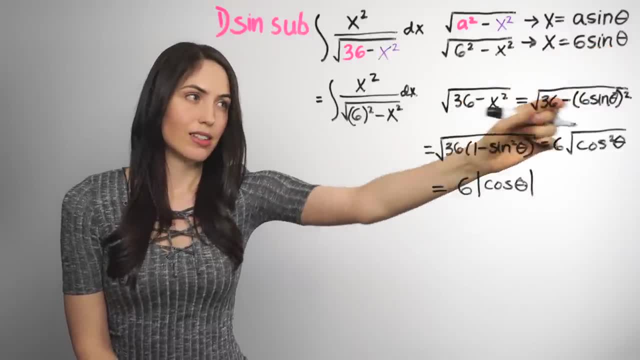 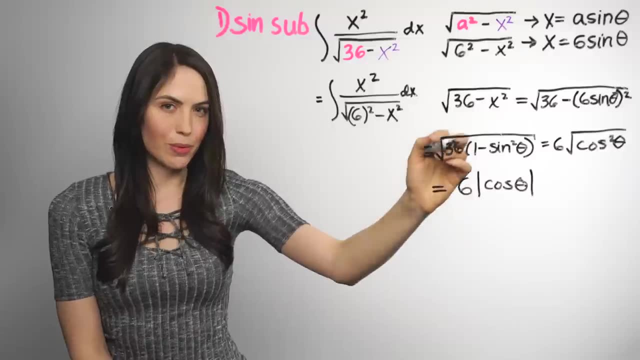 So plug in 6 sine theta for x, 6 sine theta for x and simplify So the 6 gets squared. We have a 36 from both terms. we can factor out This can be factored out front as a 6.. 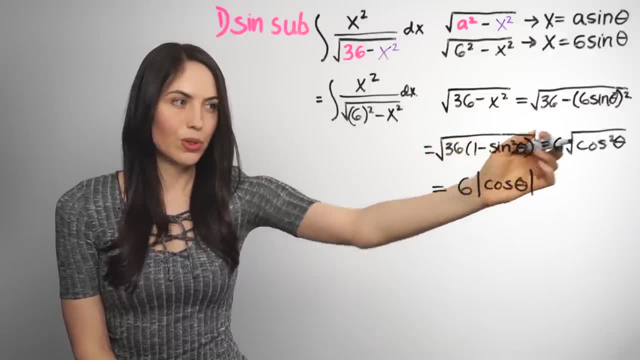 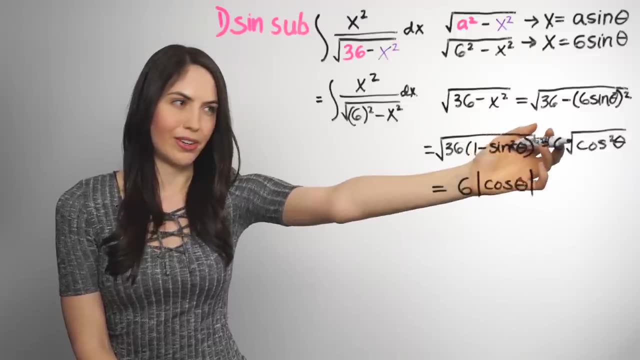 And the 1 minus sine squared theta is equal to 6.. And the 1 minus sine squared theta is equal to cosine squared theta. That's a Pythagorean relationship, Pythagorean identity. So use that. It's very important in all of these. 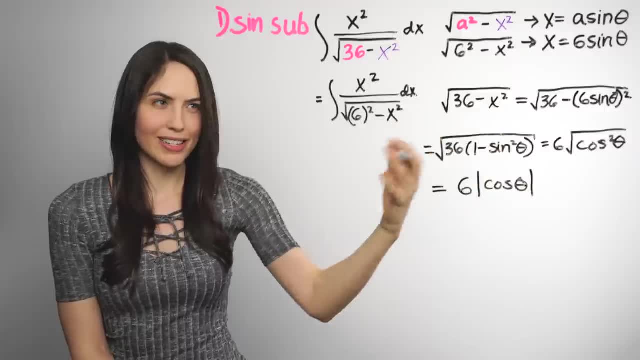 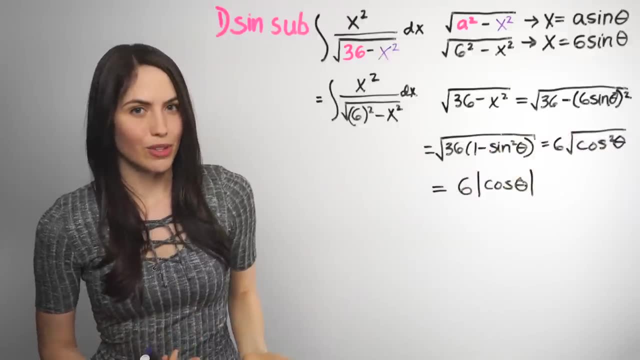 That's the key, like the real link that makes this all work. Anytime you have the square root of something squared, really the answer is the absolute value of that something. So really, our answer here is 6: absolute value of cosine theta. 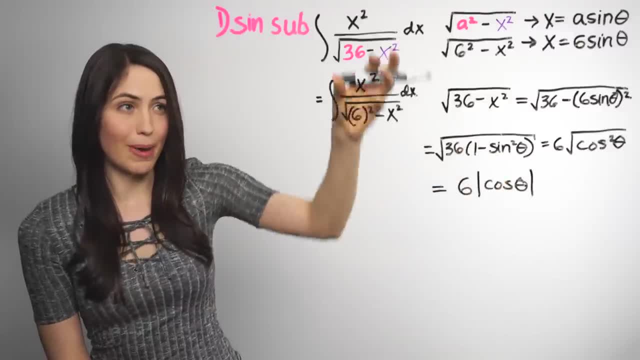 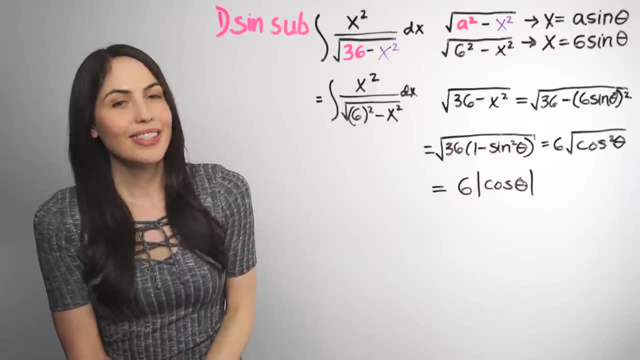 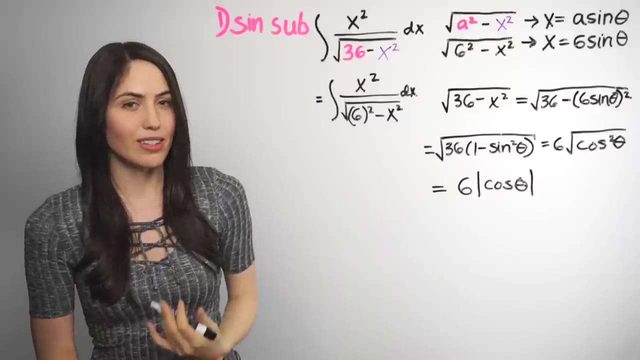 But the idea is to take this and put it back in our integral and we're not going to be able to integrate if we have an absolute value like that. So what we do for trig sub is, if we have an indefinite integral with no limits, we just assume that cosine theta will be positive. 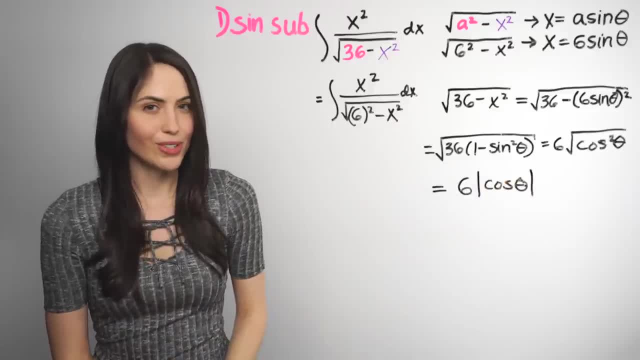 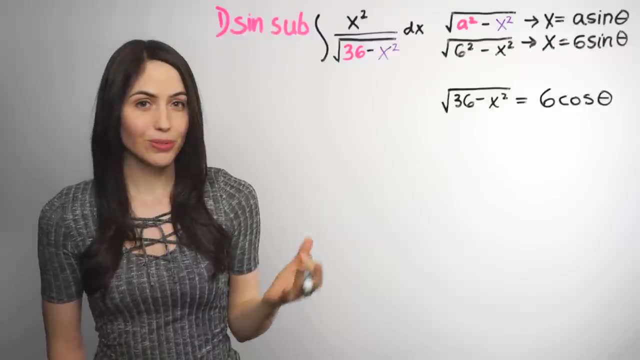 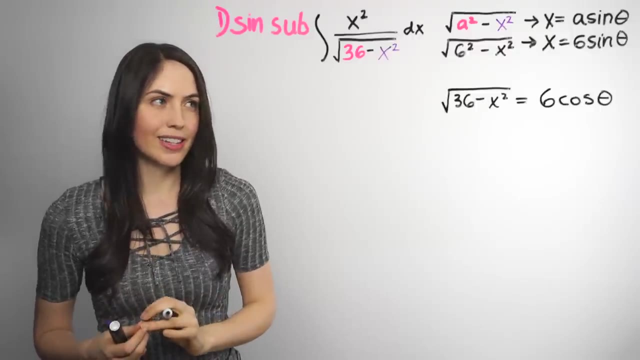 and we drop the absolute value of r's. So let's do that. So we got rid of the root with our substitution. We got rid of the root, We got rid of the radical. It's a clever trick. this trig sub the way it uses Pythagorean identities. 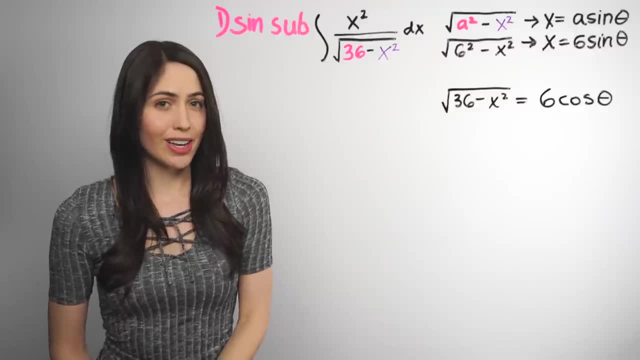 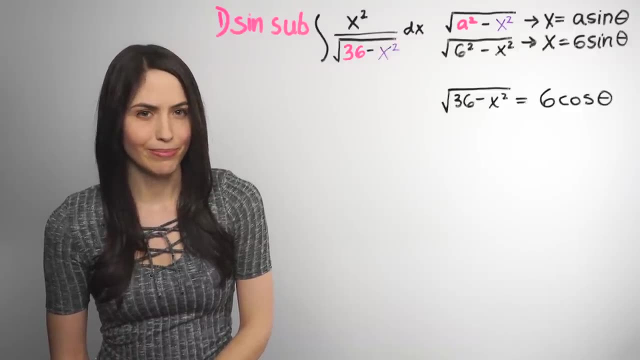 and gets rid of the radical, And I'm sure that if you had a ton of free time and the desire, you could come up with it on your own. I know I enjoy deriving new integration techniques in my free time, So we have something we can replace the radical with. 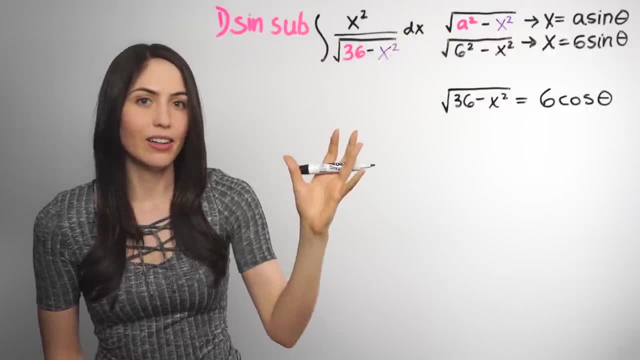 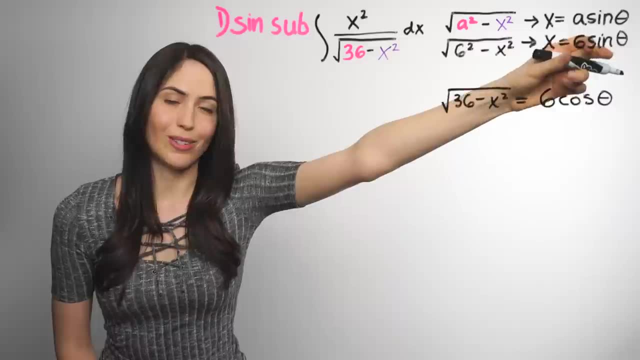 We want to replace the whole integral so that it's in terms of theta, not x. So we want to replace this x squared. We can do that. We can do that using what we know x is and just square that. What else do we need to do? 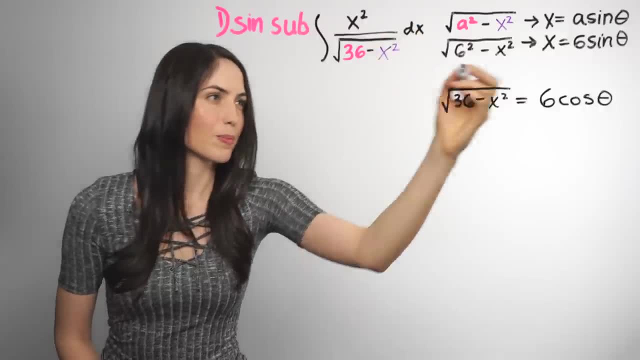 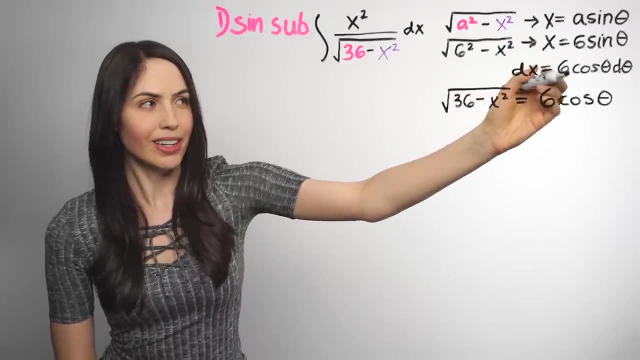 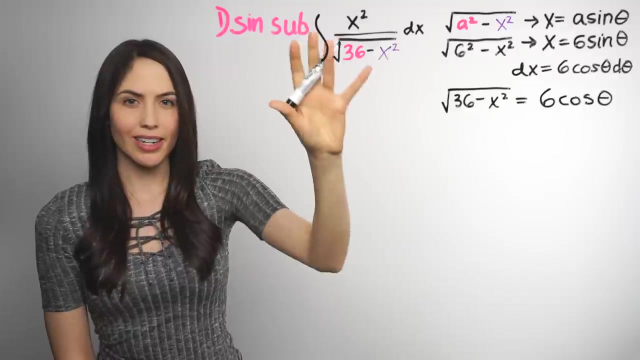 We need to replace the dx, So let's get dx. So this is our dx. we got from the x expression. I know this looks similar to the radical expression we got. That's just a coincidence. So we have our dx. We have everything. we need to rewrite this. so it's all in terms of theta. 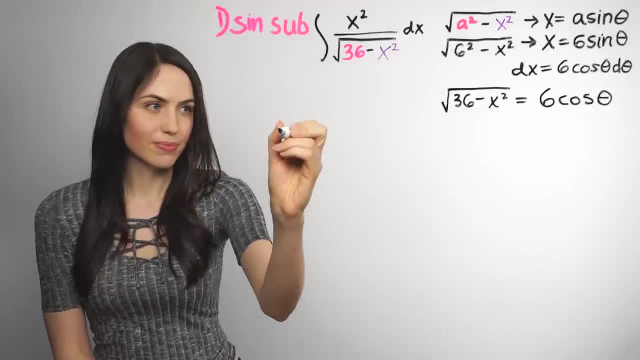 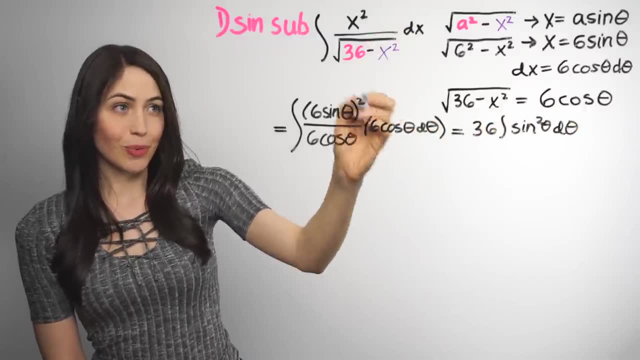 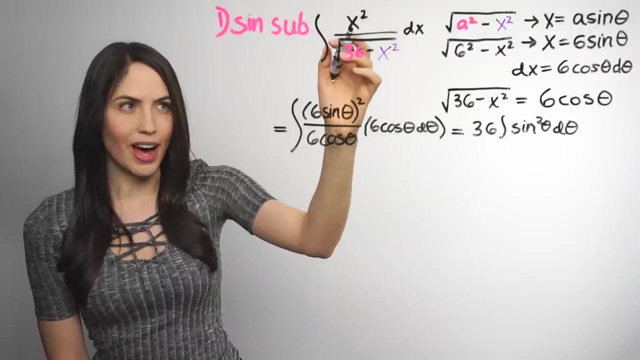 It's just the theta versions of everything. So let's do that. So we've replaced the dx, We've replaced the radical, We've replaced the x squared factor. Whatever other leftover x factors, you have replace them. So the x squared, even if the x squared were down here. 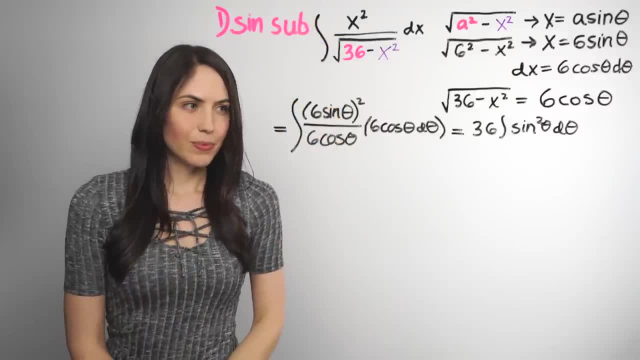 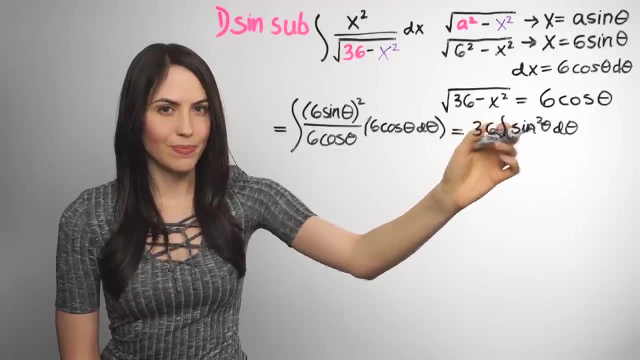 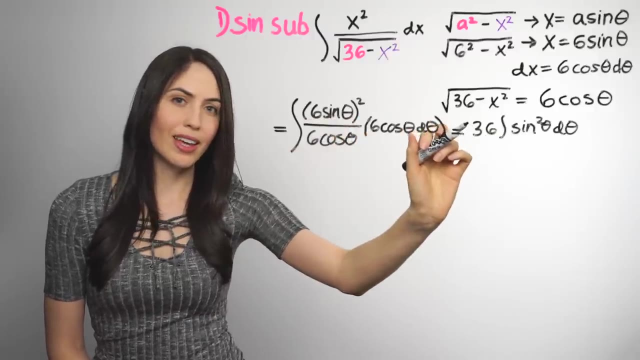 Whatever you have, replace those x's and clean it up. So when we clean it up, we get 36 times the integral of sine squared, theta, d theta. And listen, guys, At this point, when you have trig substituted and cleaned it up as much as you can, you. 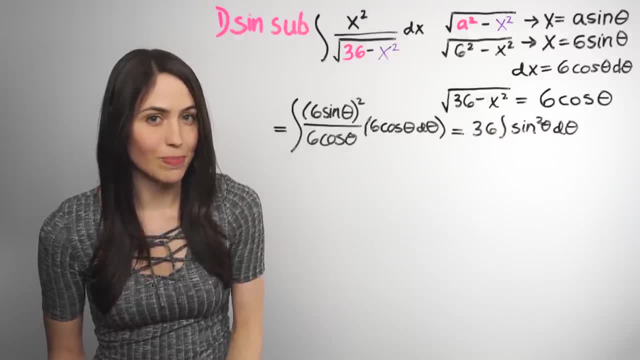 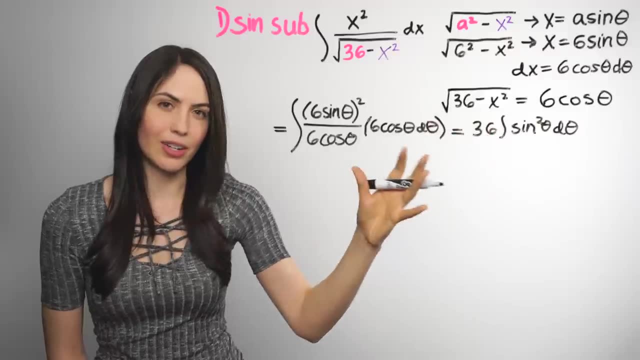 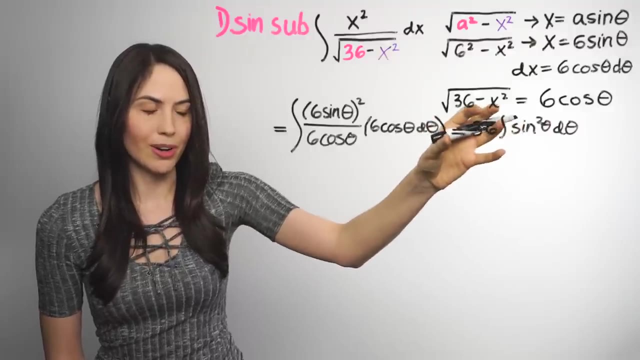 need to pull out your best integration skills that you've been buffing up, hopefully, and use them to attack the integral with everything you know about integrating trig functions, Because this is no longer unfamiliar territory, This is no longer trig sub territory, This is general integration territory. 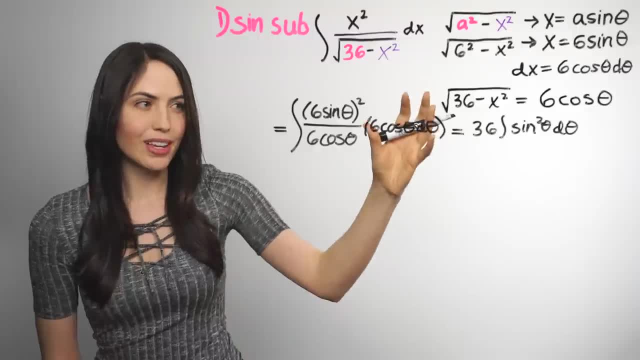 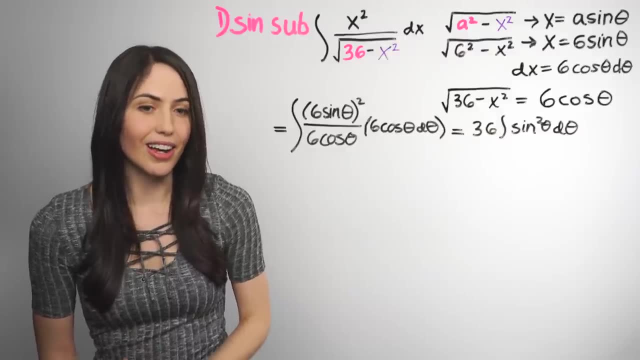 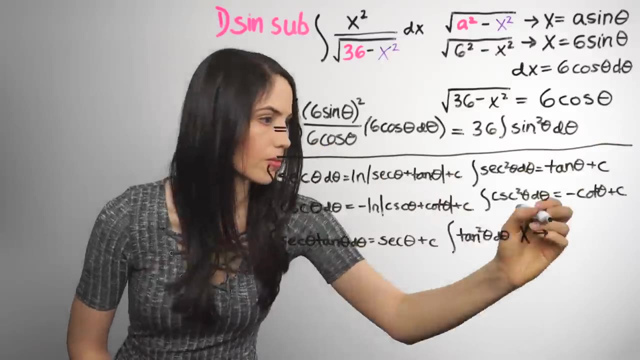 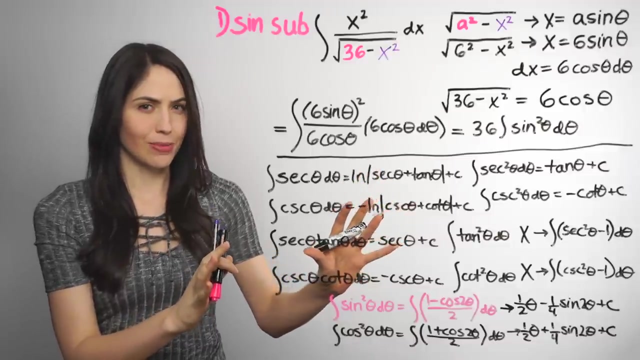 So use everything you know about integral rules, trig identities, algebra tricks to integrate it. But because I care and I feel your pain, really quickly, let me help you out a bit. All right, These are all really common outcomes of trig sub, so I know this is a bit of a cluster. 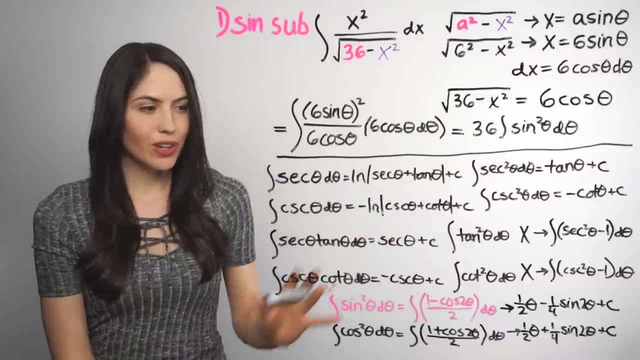 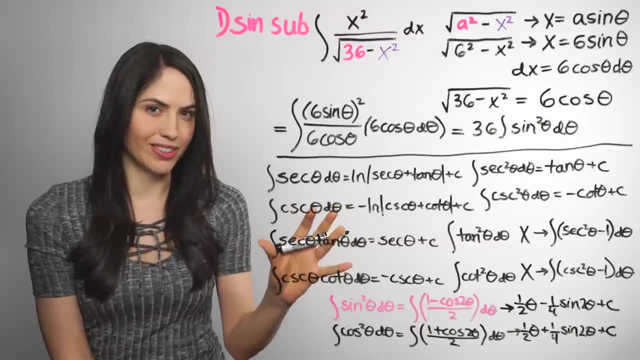 fuck, This is more than you would ever ask for, But these are all really common ways it could turn out when you do trig sub, where you will need an integral rule from the table of integrals to integrate. It's just good to see them so that you're familiar with what you can do. 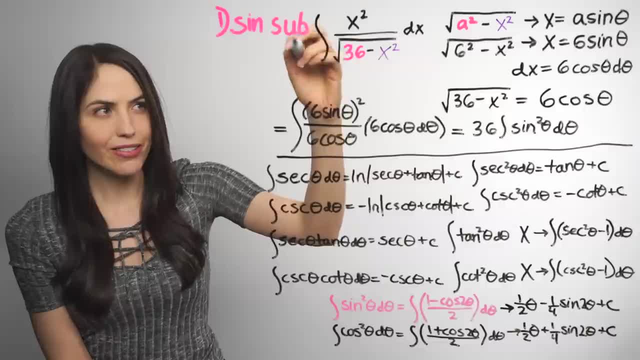 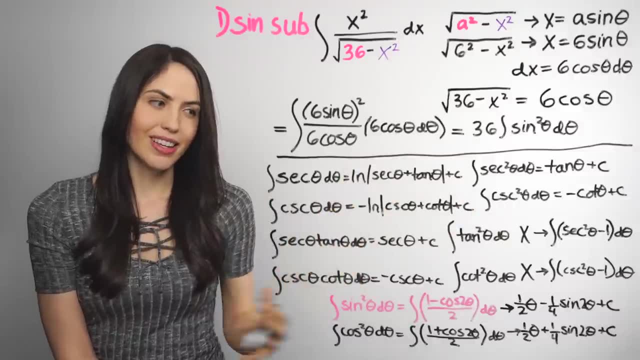 It all depends on what you were given, like the specifics of your original integral, Instead of getting the integral of sine squared. you could just as easily get one of these, And you will run into all of these if you do enough trig sub problems. 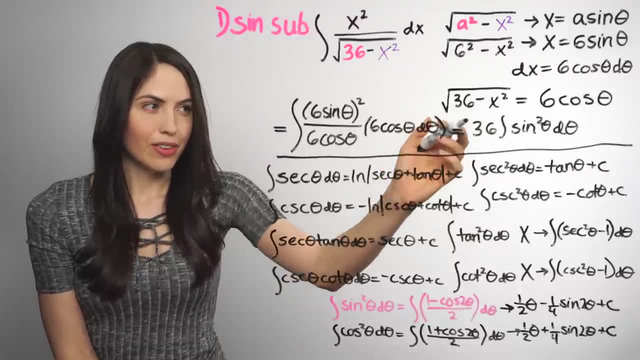 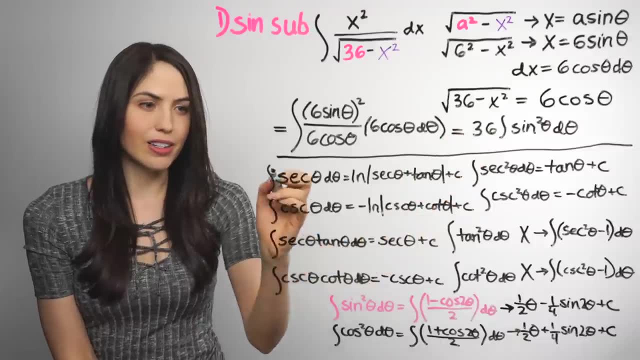 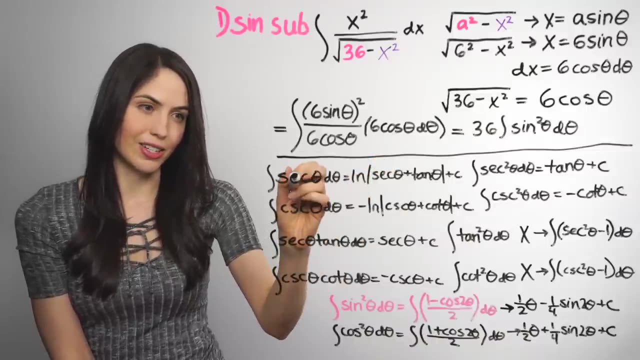 But Save it instead of the integral of sine squared theta after you substitute it and clean it up. Instead of that, if you got the integral of secant, for instance, you can use the integral rule from the table of integrals, the secant integral rule. 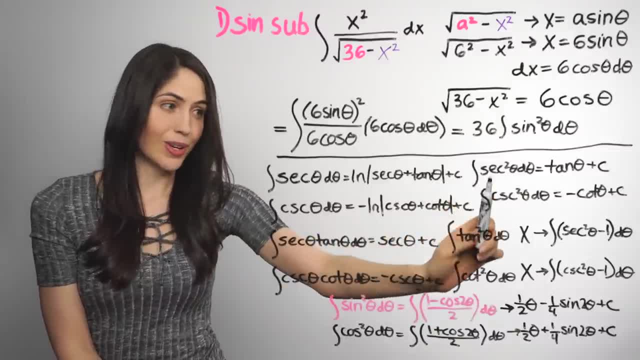 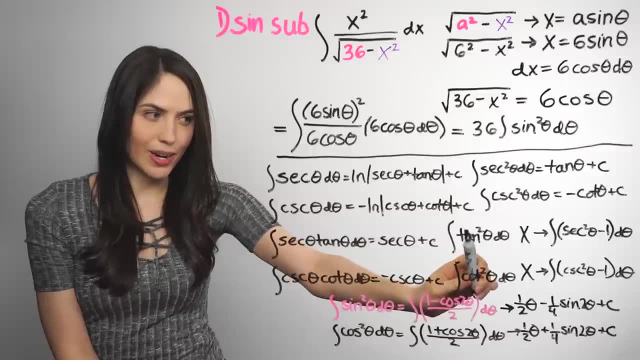 Or cosecant has one integral rule. Secant squared has one. Cosecant squared has one Integral of tangent squared. there's no integral rule for that, but you can replace tan squared with secant. Secant squared minus one. the Pythagorean identity. 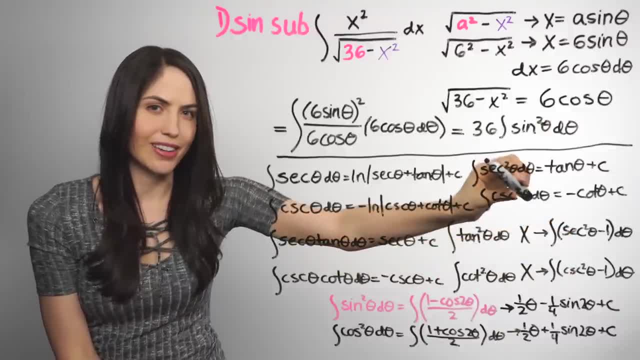 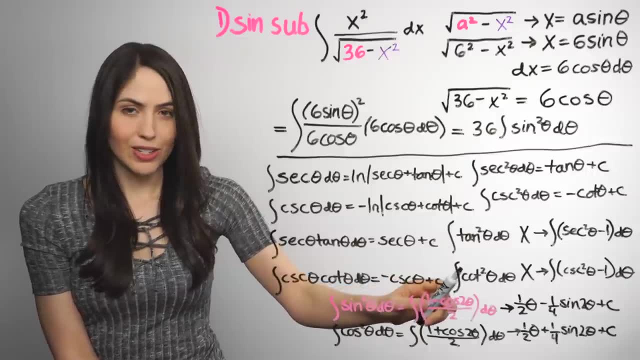 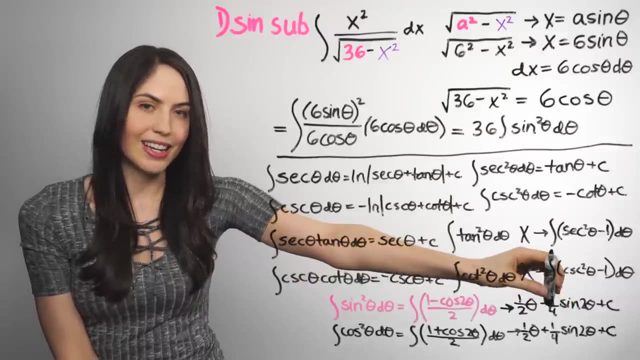 And then use the integral rule for secant squared. This is a common one, you might see. Here's the cotangent squared version. There's not a rule straight away, but you can replace it with the Pythagorean identity And then use the integral rule for cosecant squared. 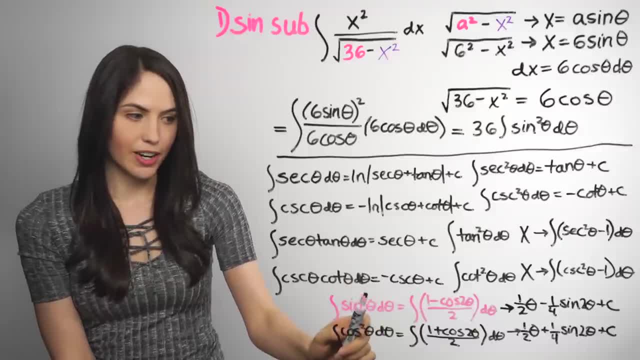 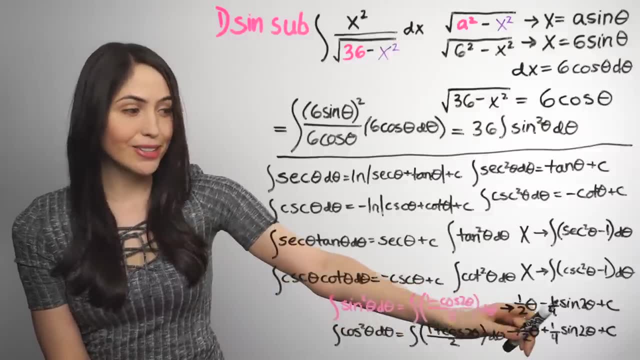 This is ours. This is what we're going to need. Integral of sine squared. Integral of sine squared. Is there a rule on the table for that? Maybe, if you're lucky- depends on your table- you might be able to use this straight away. 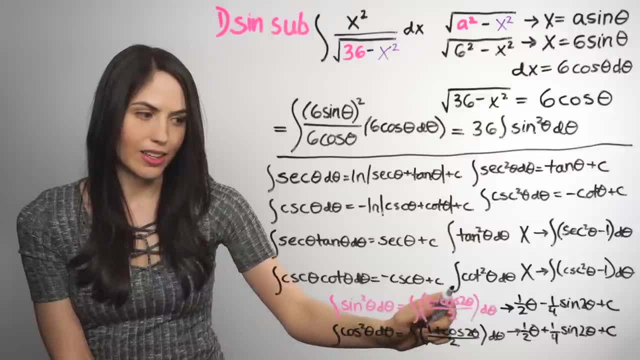 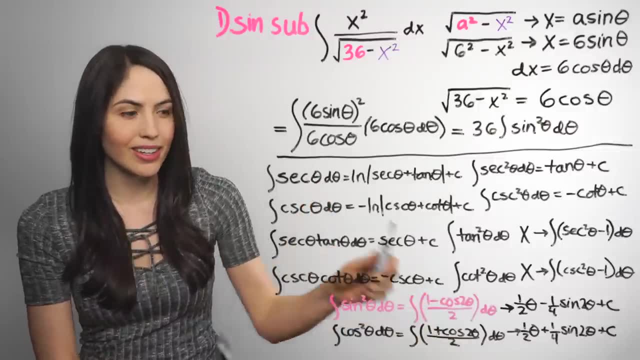 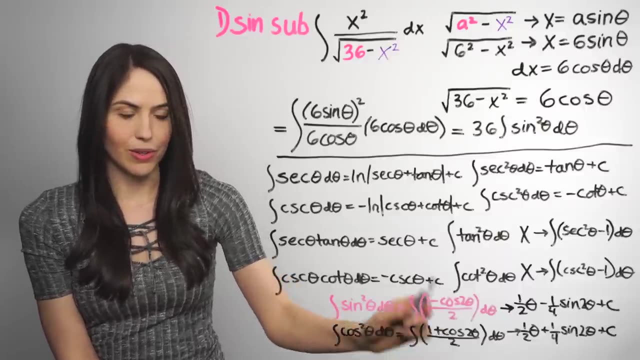 More likely. you have to replace sine squared with a half angle identity. It's a trig identity, also known as a power reducing identity, And once you've done that, you can integrate that. This is the cosine squared version of that with a half angle identity. 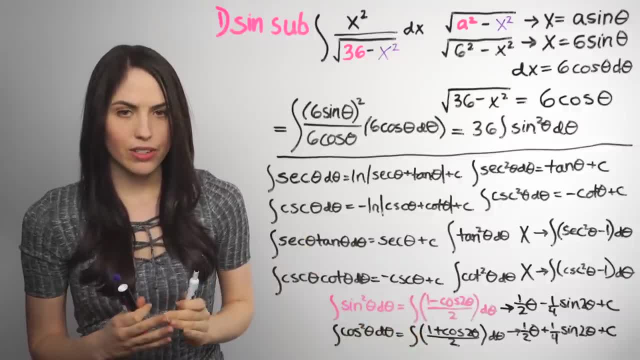 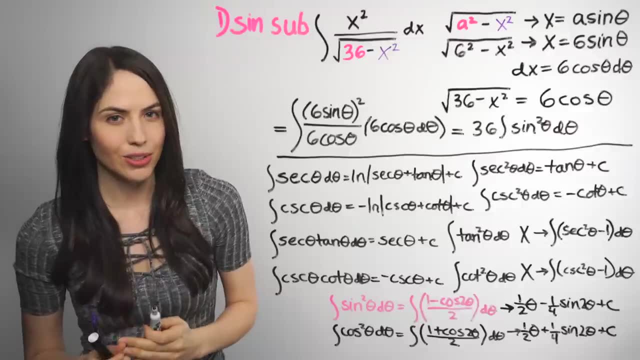 For it. And if you get one that's different trig functions, multiplied and divided but with powers, there's a good chance you might need something called trig integral rules. More on that later, if you don't already know what I mean by that. 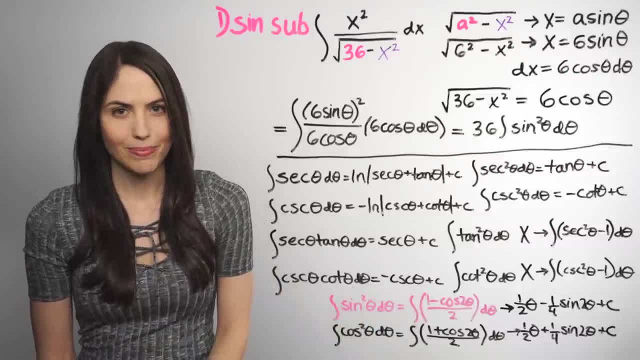 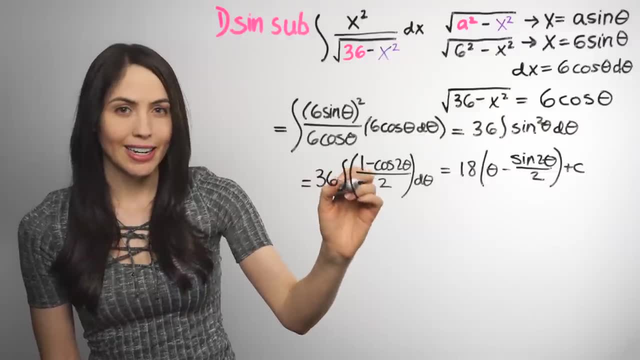 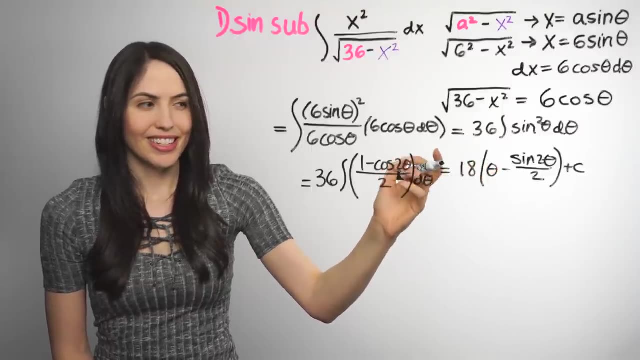 But let's use this one for ours: the integral of sine squared theta. Okay, so we used the half angle identity and then we integrated. we have an answer for the integral Great, But it's in terms of thetas, it's not in terms of x's. 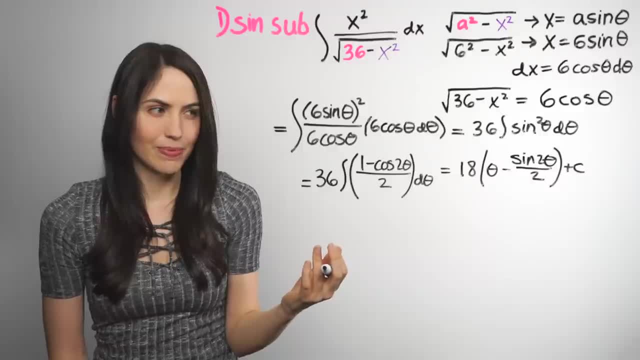 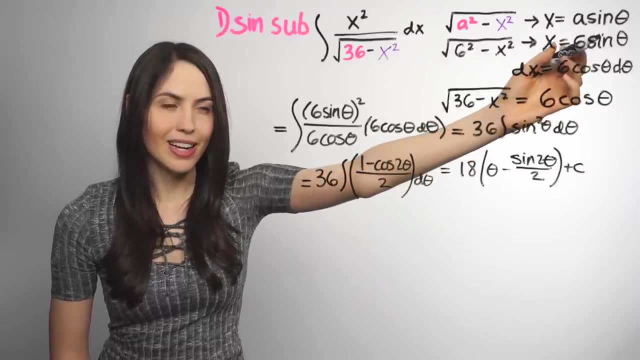 We have to get back to all x's for the answer. So how do we convert it back to all x's? We can use our substitution: x equals 6 sine theta. Right now, this is sine of 2 theta. If it were sine of theta, we could use this: 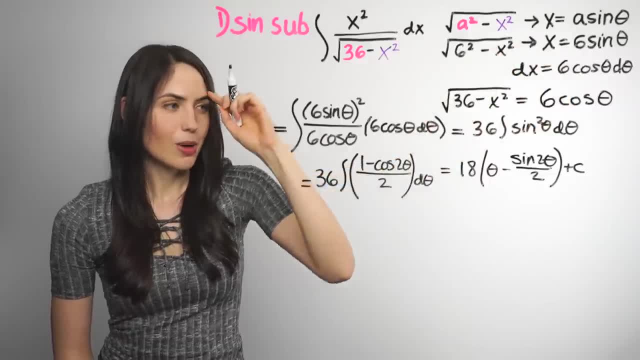 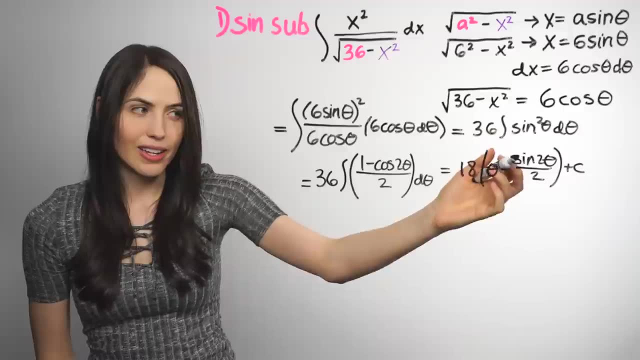 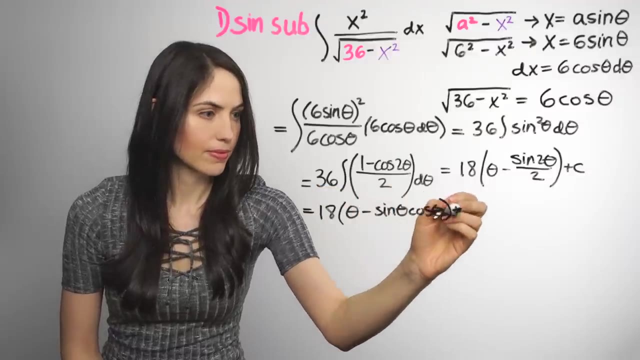 Sine of theta would be x over 6, and we could substitute that We have sine of 2 theta. so what do we do with that? When you see that use the double angle identity Sine of 2 theta is 2 sine theta, cosine theta, so rewrite it with that to simplify. 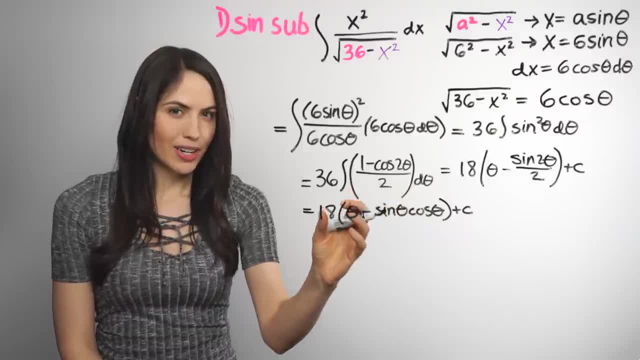 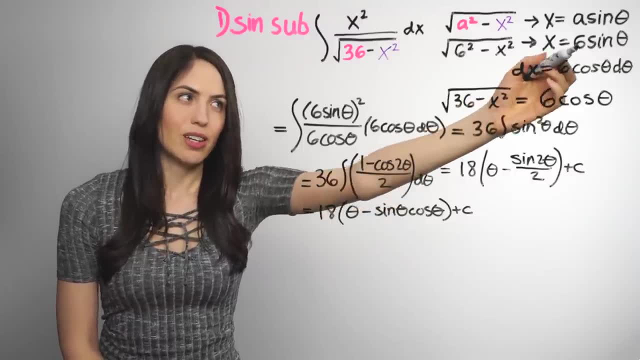 So now let's rewrite this in terms of x substitute in x expressions, where we can, For sine theta. we do know what that is in terms of x. because of our substitution, Sine theta would be x over 6.. Great, Thank you. 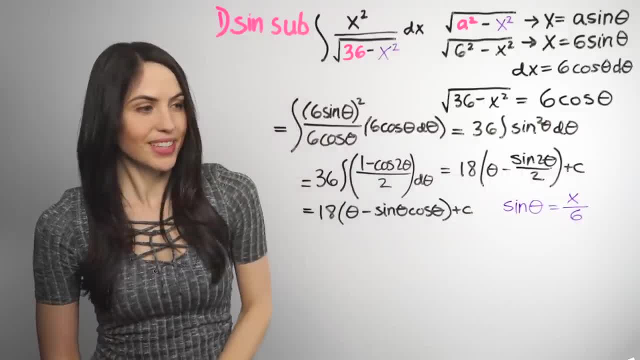 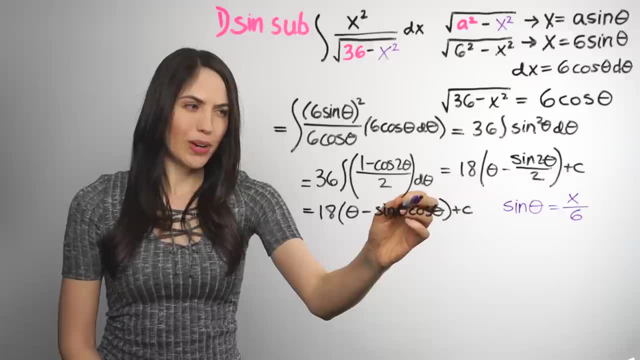 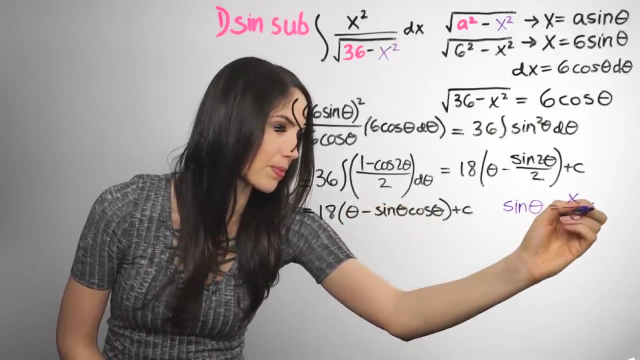 Bye. So we can use that for sine theta to replace that in terms of x. But how do we replace cosine theta? We don't have that already. How do we get it? We have to do a little bit of right triangle trig. 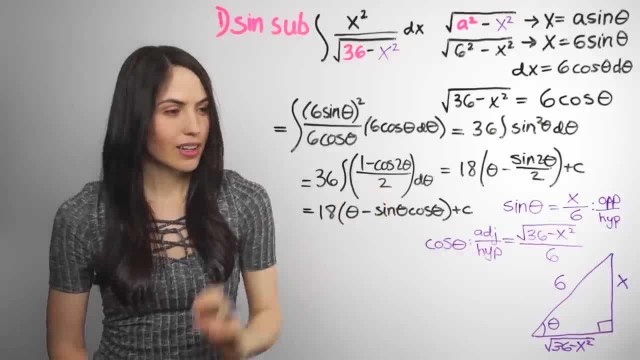 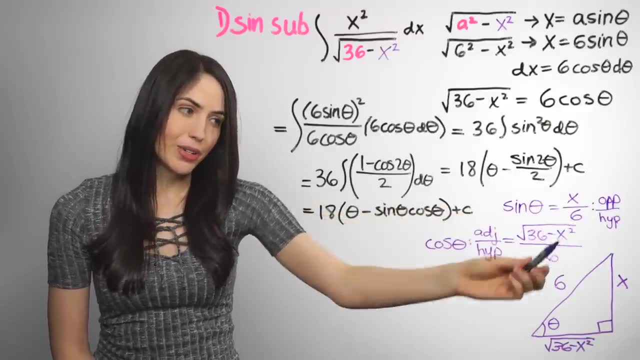 So with the right triangle we can get any trig function we need. So because we knew that sine theta is x over 6.. x over 6, and sine theta is opposite over hypotenuse. If we draw a little right triangle and sine of theta is: 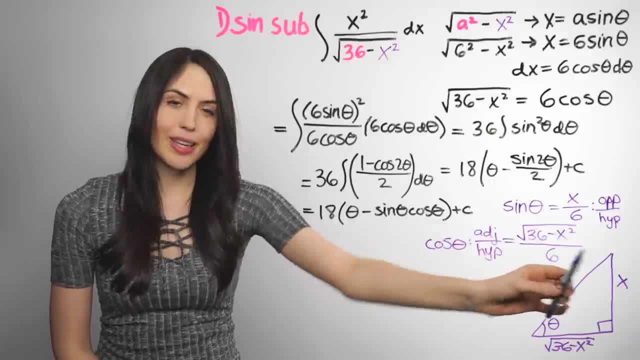 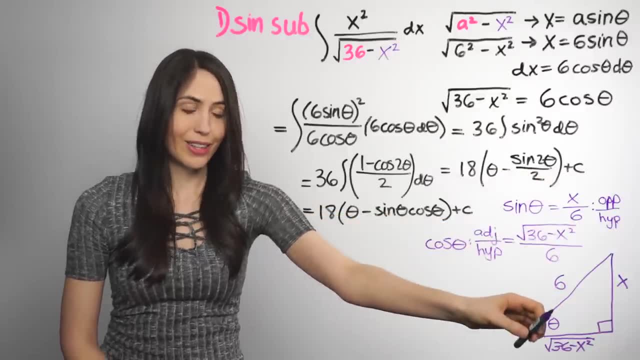 opposite, over hypotenuse x, over 6, we can label those sides. And once we've labeled the sides, using sine, what we know for that, we can find the third side with the Pythagorean theorem, your friend, the Pythagorean theorem. 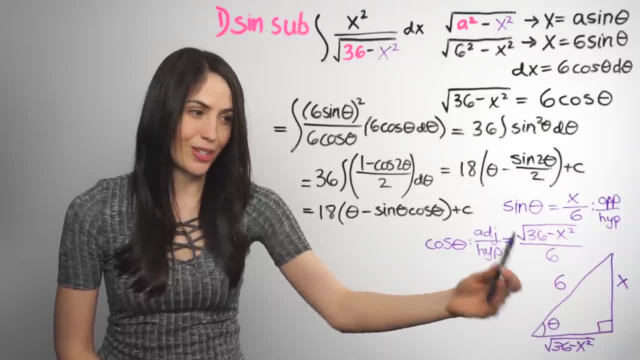 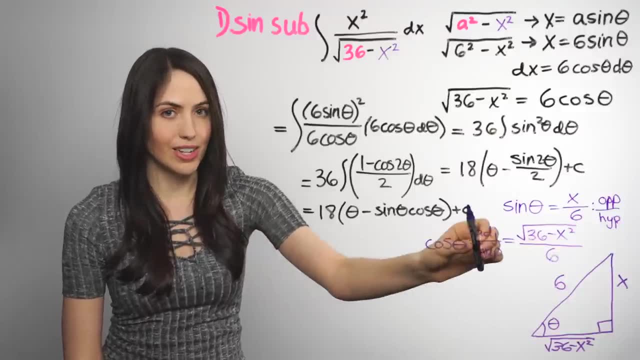 And it ends up being the square root of 36 minus x squared, which should look familiar. Now that we have all the sides, you can get any trig function that you want. like cosine is adjacent over hypotenuse, So it will be this root over 6.. 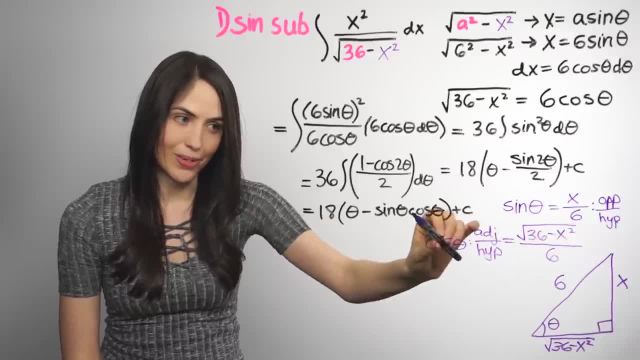 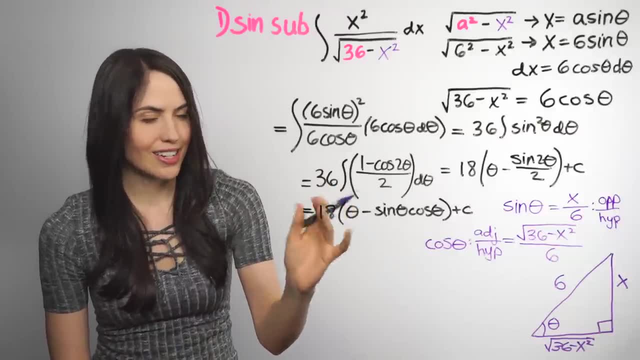 So that's our cosine that we can plug in. It's an x expression for cosine We can plug in, for that Seems like we should be done, but there's this theta left here by itself, And we can't just leave it like that. 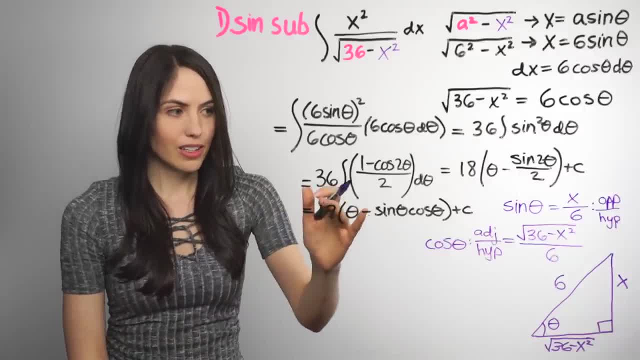 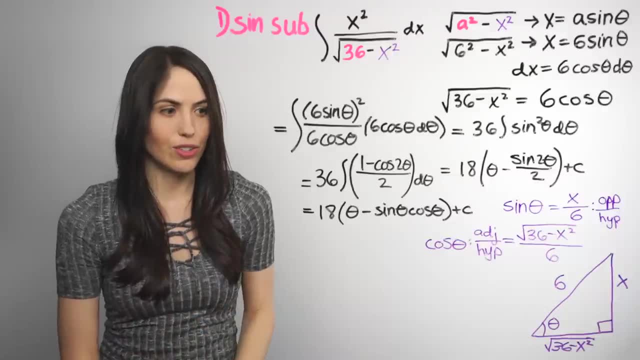 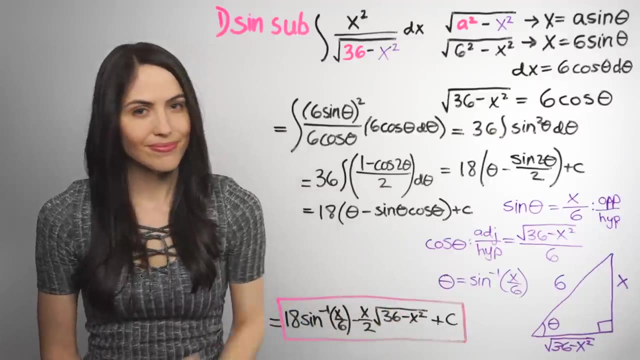 So how do we do it? Well, if you see one like this, you can take any trig function you have, like sine theta, It's x over 6. And just use the inverse trig version of it to get theta alone. OK, so if you plug all those in, plug in for cosine theta, sine theta. 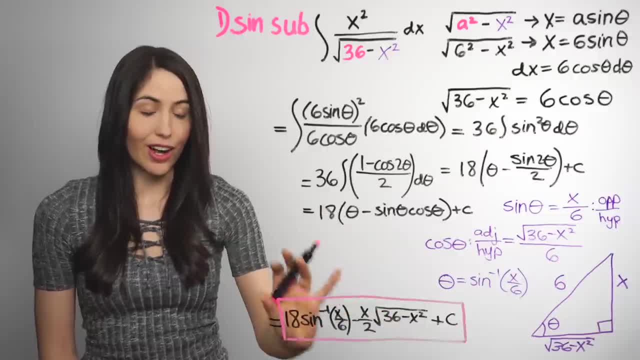 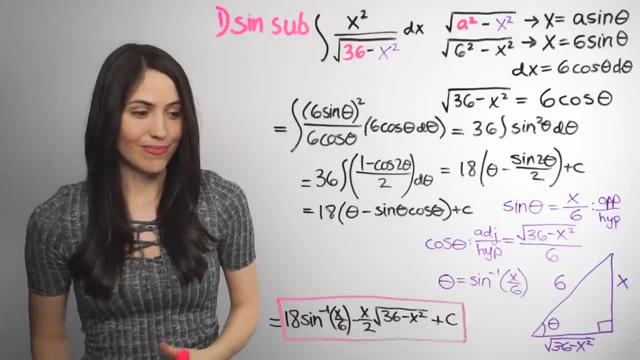 theta and simplify, you'll get this. It's all in terms of x. That's the answer for the integral. So that was sine substitution. It's a lot of work, huh, It's a lot of work to explain everything. 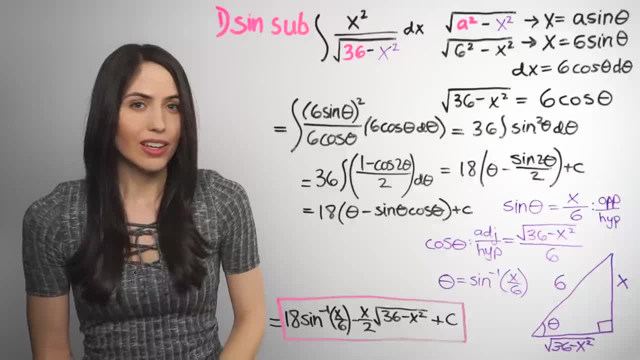 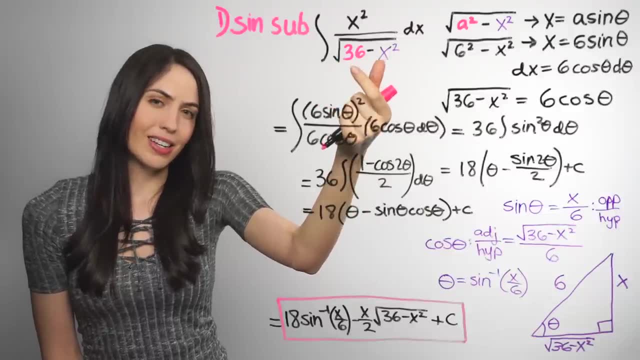 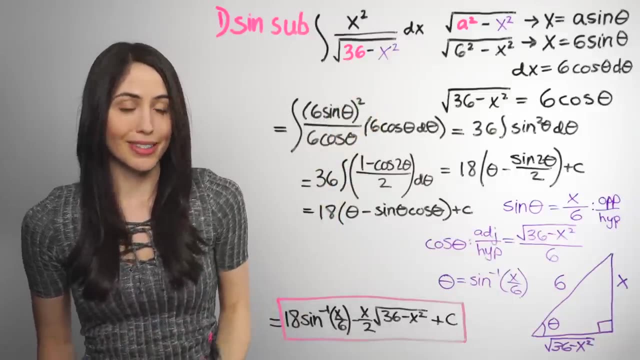 We'll be faster next time. Keep in mind, if you had one that was actually x squared minus 36 under the radical, like the reverse of this, that form would be secant. substitution: a different type of trig sub That's coming up. 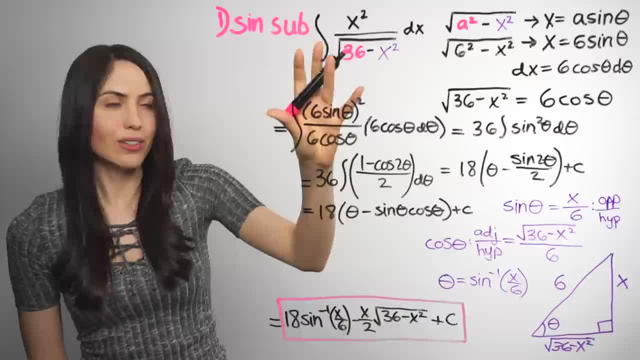 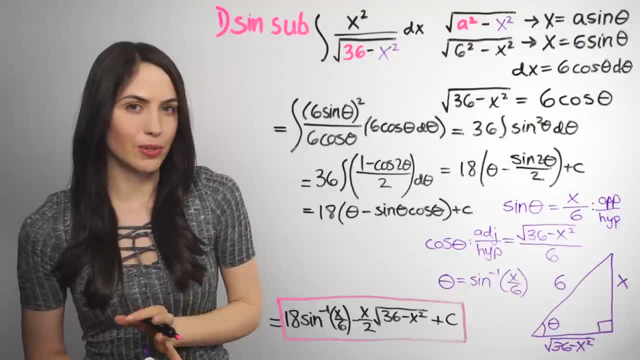 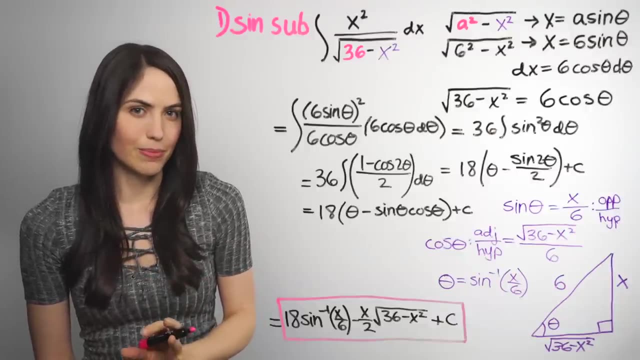 Also, if you see one that's like this, has a radical, looks like this, but you know you can do u substitution or you know you can do an integral or you can do an inverse trig integration rule. even then you can do trig sub if you want to. 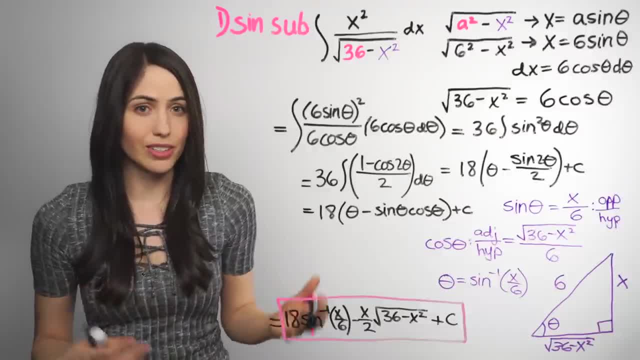 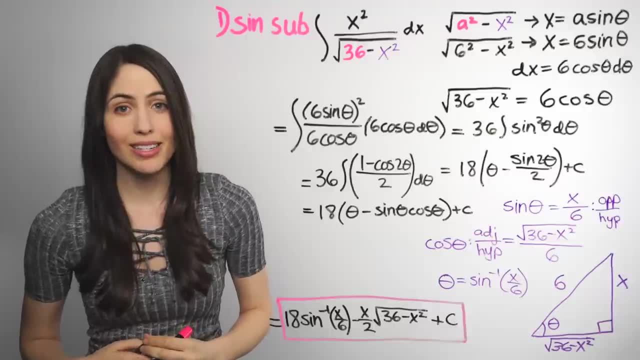 If you have to, or if you just want to, just to be different, go rogue, do your own thing and not be part of the lockstep masses. You can if you want. It may not be the easiest way to do it, but it will work out. 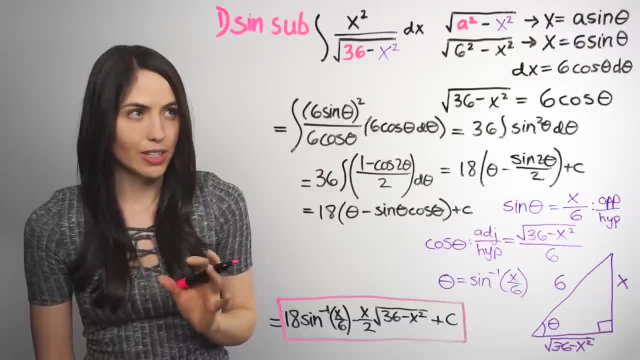 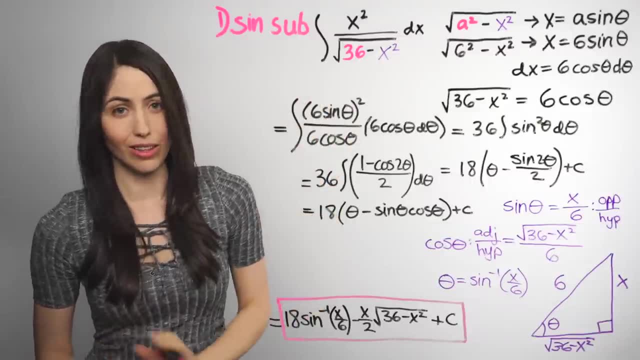 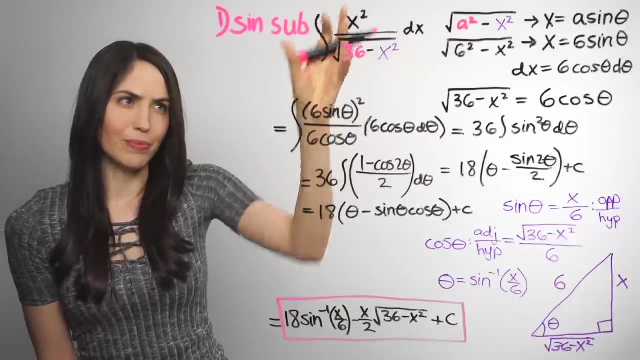 Sometimes you have a choice that way, And trig substitution is just a technique to get the integral OK. It's not the law to integrate the integral into a form that you can integrate, It's not the law. What would you do if you had one with a radical up top in the numerator though? 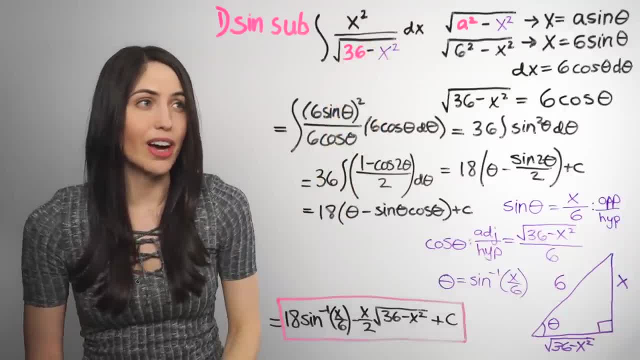 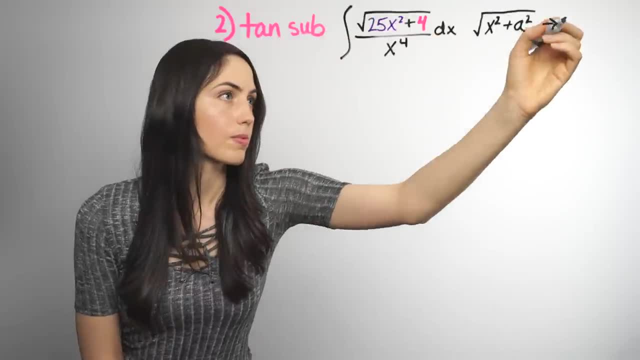 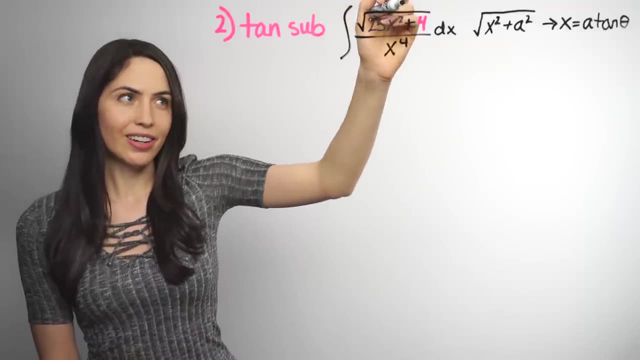 Or if you had a coefficient on x squared, like 4x squared, 9x squared, 25x squared- How would you do that? Or when you have both, if you have a root up top in the numerator and some coefficient. 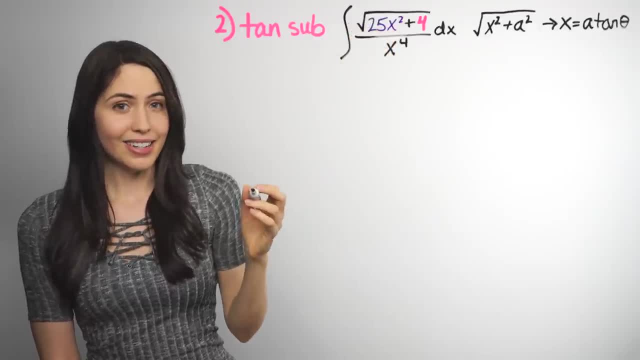 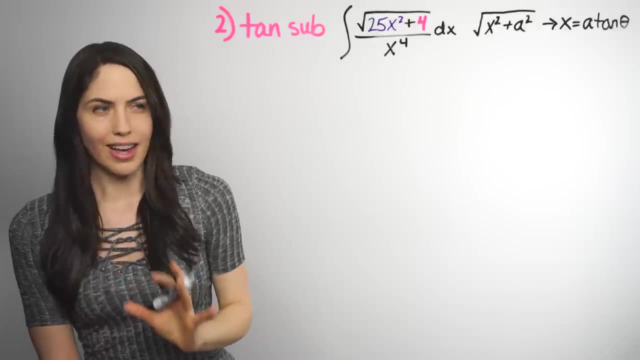 on the x squared term and if you have addition under the root, so if you have a plus here under the radical, what do you do then? I know this seems a little disastrous, but don't worry, I will show you how to do it. 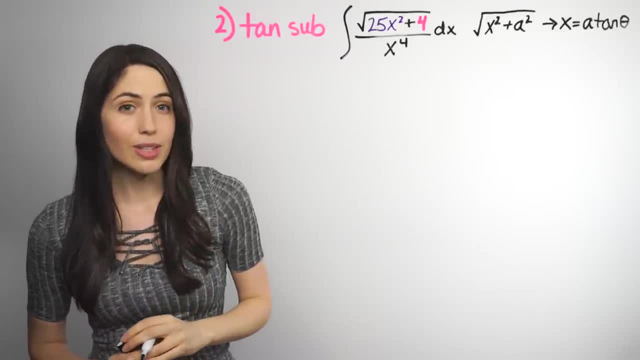 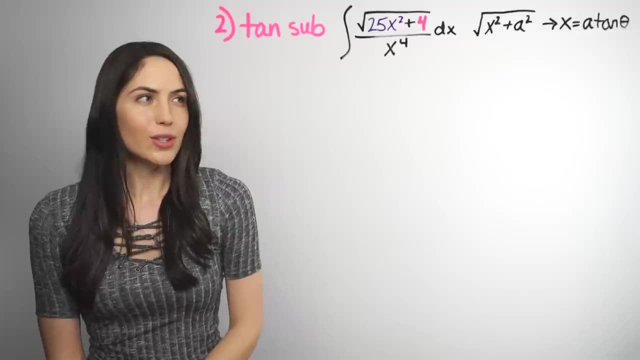 Just first, though, you should technically check to see if you can do something like u substitution Or use an inverse trig rule to integrate. You can't, It won't work out here. So let's see if we can get rid of this root using trig substitution and then see if we 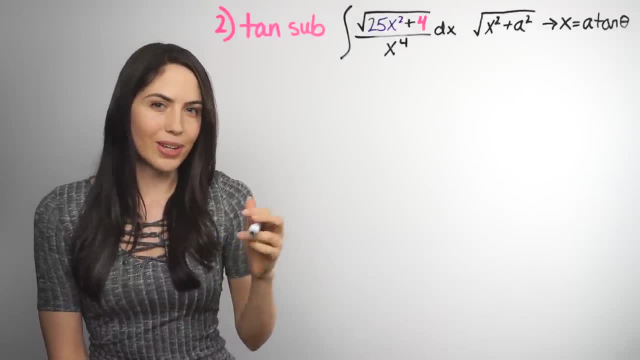 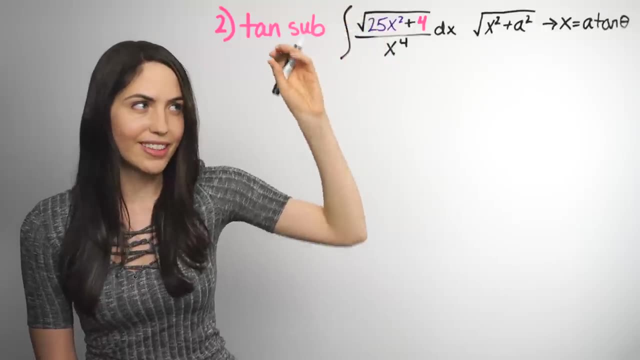 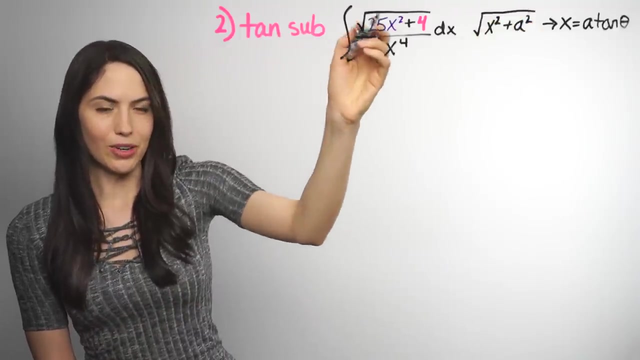 can integrate. So I know I said earlier that when you have an x squared term plus a constant squared under your root, that version, that it will be the tangent type of trig substitution, And it will be. But what do we do with this coefficient here? 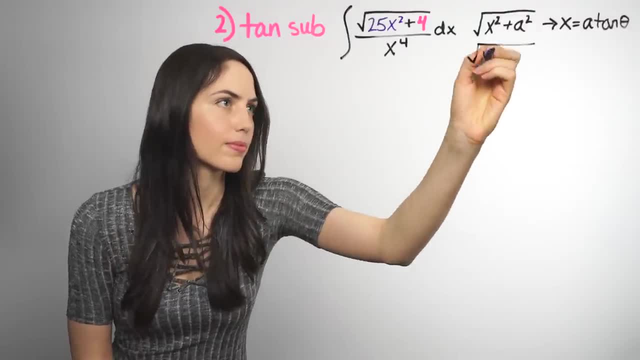 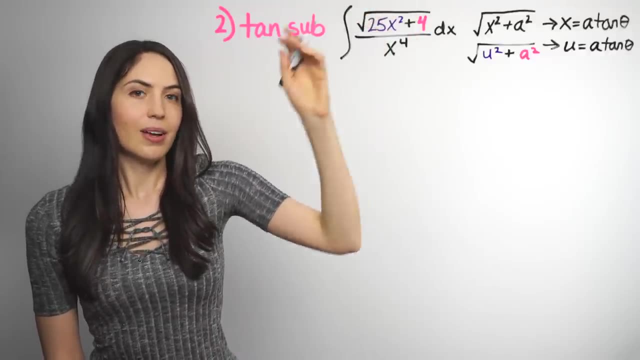 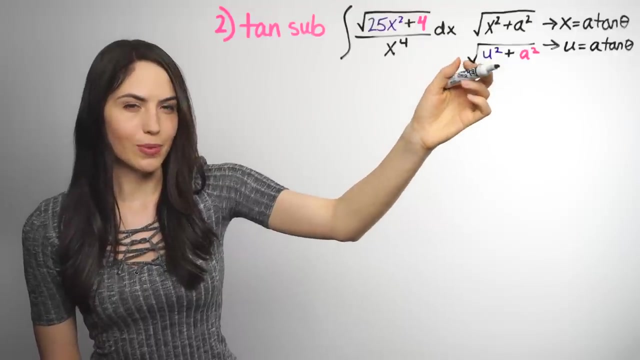 We'll just use the 25.. So when you have a coefficient on x squared in the radicand, instead of thinking of it as x squared plus a squared, you can think of it as u squared plus a squared, So you might see a? u. 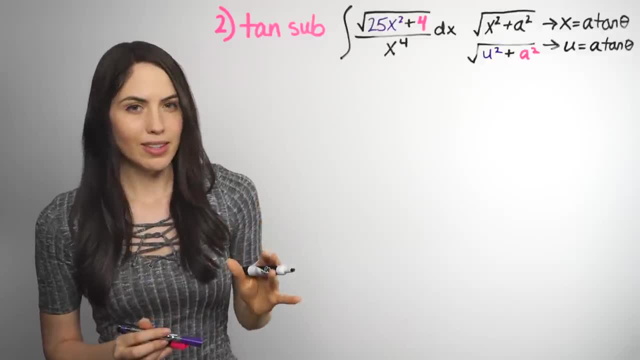 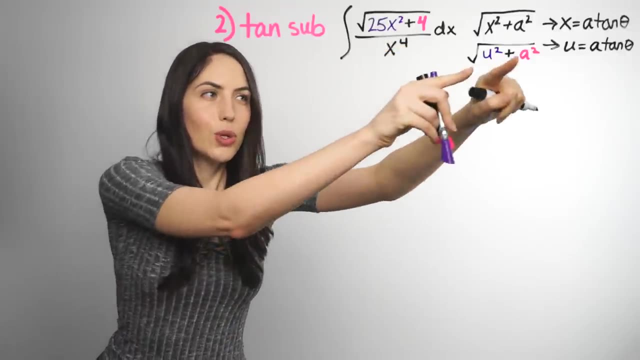 Some people use u. There are a few different ways of doing this kind, but no matter how you do it, the idea is to rewrite this as u, So you might see a u. Some people use u. Some people use a squared. 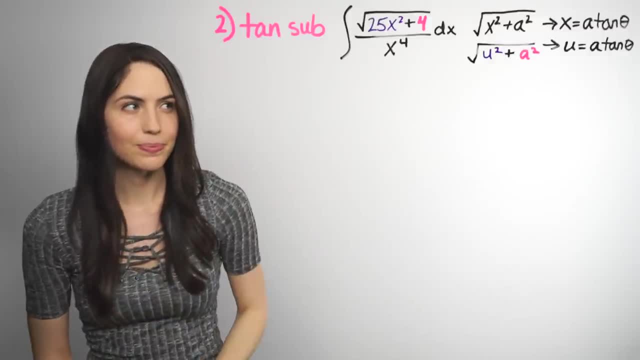 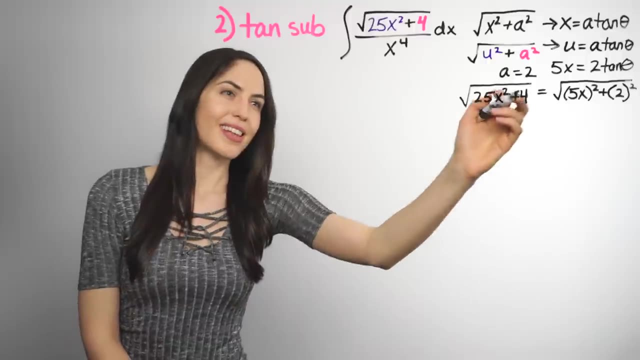 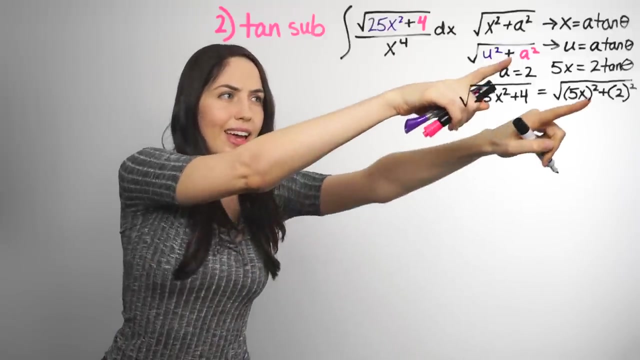 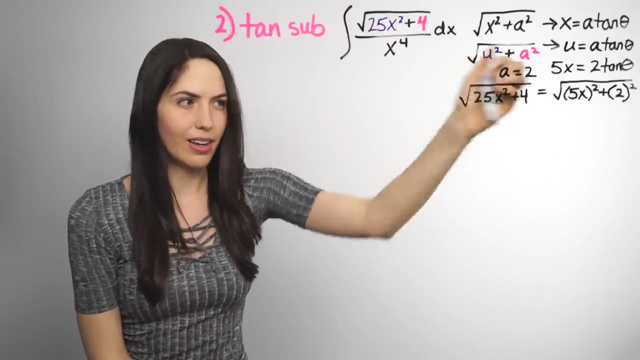 Some people use a squared But we have two things squared and added together. So when we rewrite this as one thing squared plus another thing squared, we can see that definitely a is 2.. a is 2. And u will be 5x, because 5x squared was 25x squared. 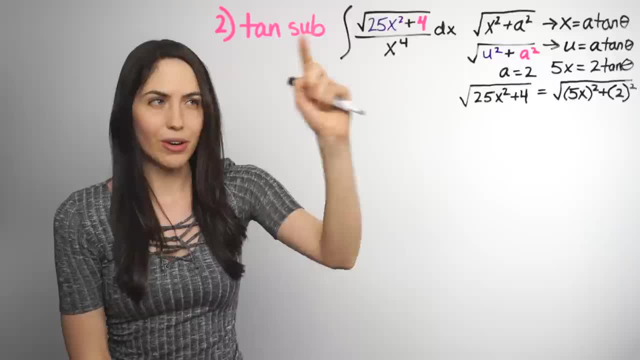 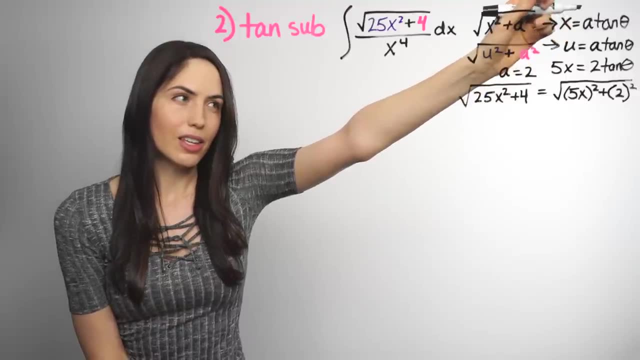 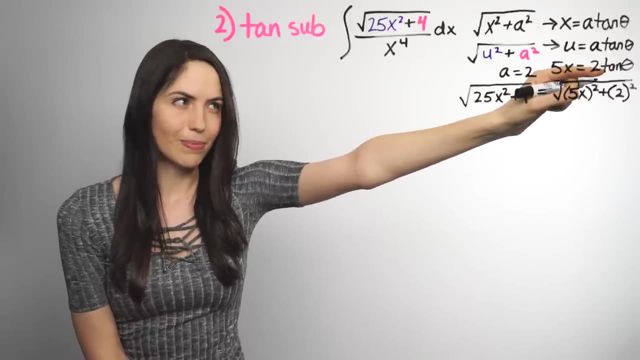 So u is 5x For this kind when you have a coefficient on x squared. basically, what you do is, instead of using x equals a tan theta for your substitution, use 5x, the u the thing getting all squared equals a tan theta for your substitution. So for us it's 5x. 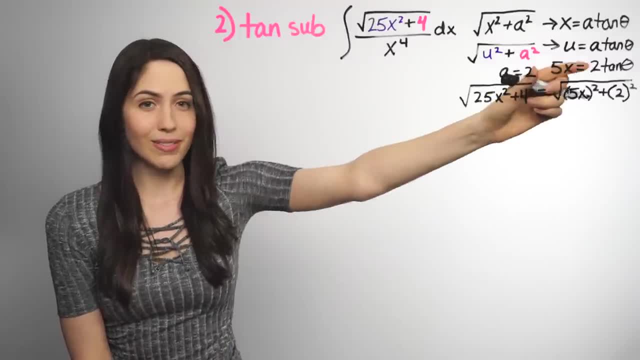 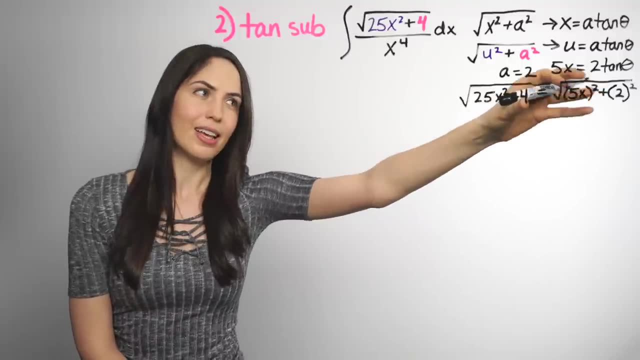 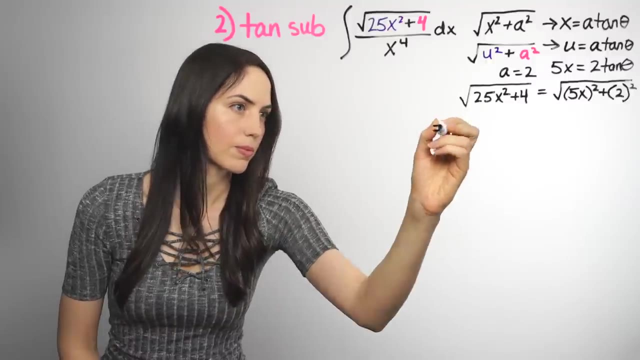 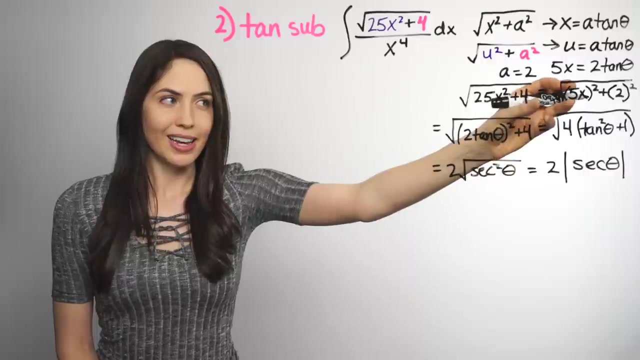 equals 2 tangent theta. That's our substitution. That's great, We have that. And now, just like before, take just the radical. out the radical and plug in your substitution and see how it simplifies. So now just use algebra and plug in, Use the substitution, plug in for 5x simplify. 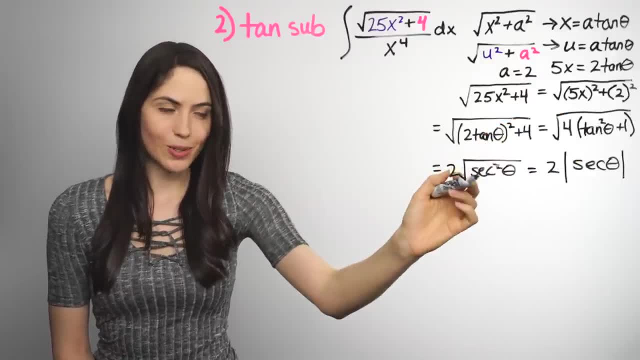 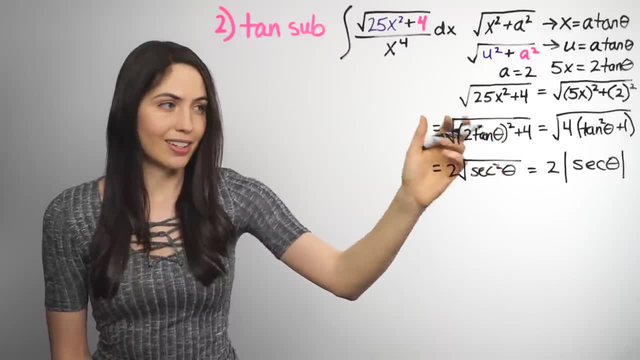 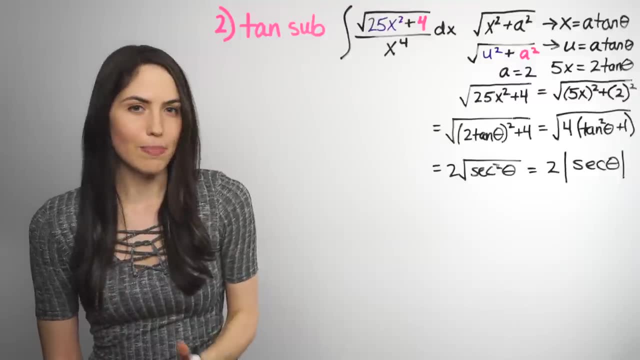 The Pythagorean identity magically breaks down the roots and leaves you with just 2 times the absolute value of secant theta And, just like before, we can drop the absolute value bars because we're doing an indefinite integral and we'll just assume everything's. 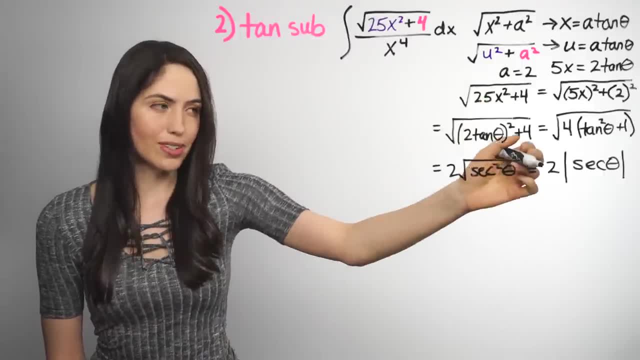 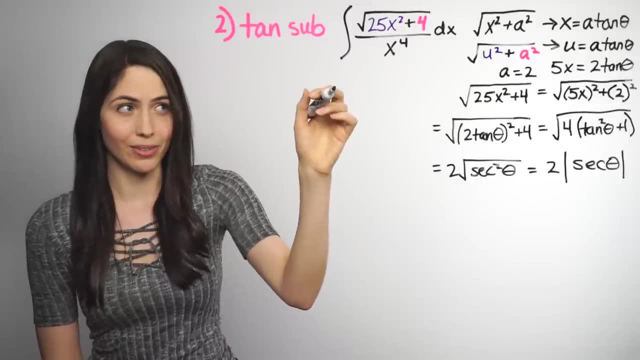 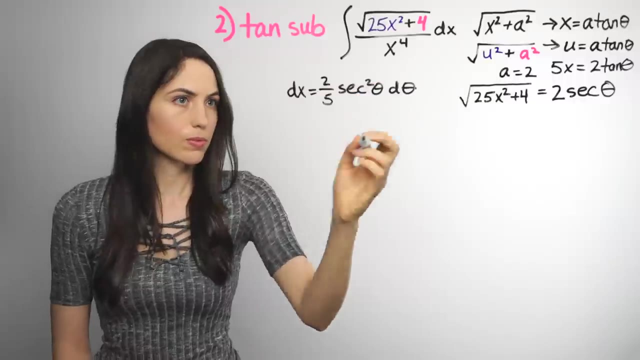 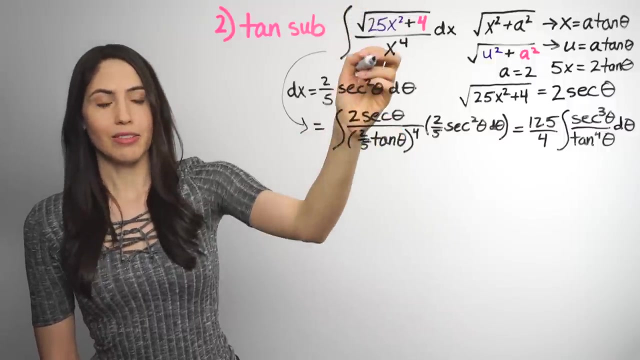 positive. So really this radical is just equal to 2 secant theta. So let's use that to replace the radical up here and replace everything else in the integral, including the dx, Don't worry about that. Okay, we plugged everything in. Plug in for the radical, plug in for x to the 4th use. 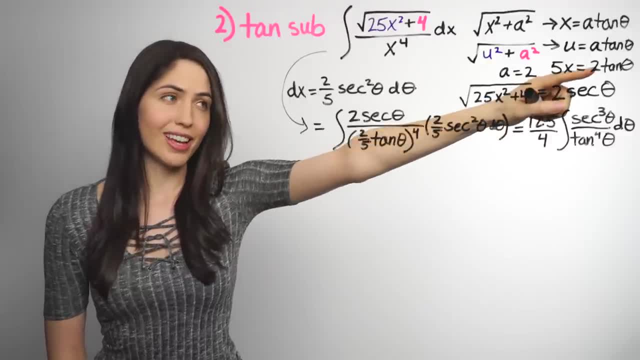 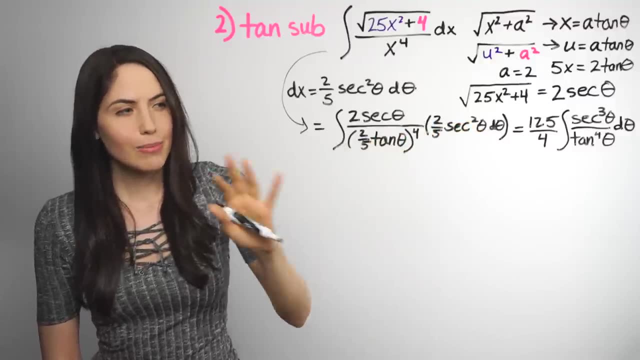 what we know. x is x would have to be 2, 5ths, tan theta. so that gets all raised to the 4th power. This is dx. And then just clean up the debris of that trig substitution and you get this which you now have to integrate. 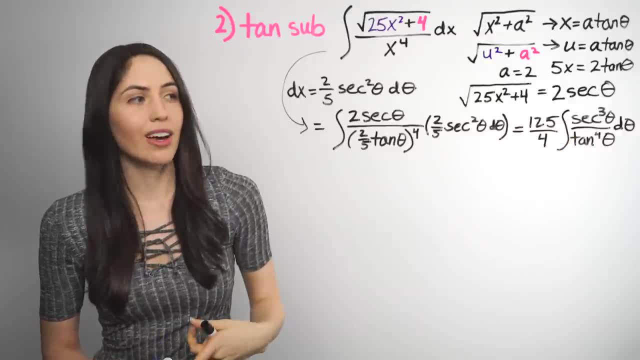 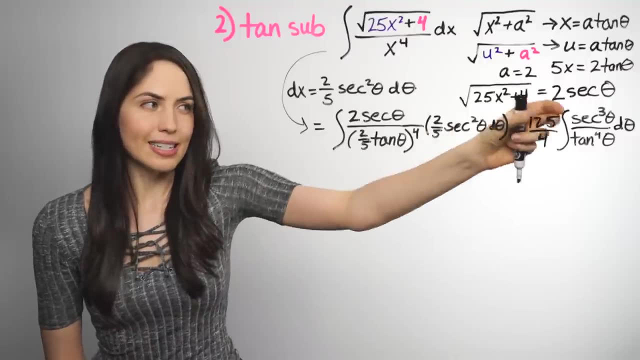 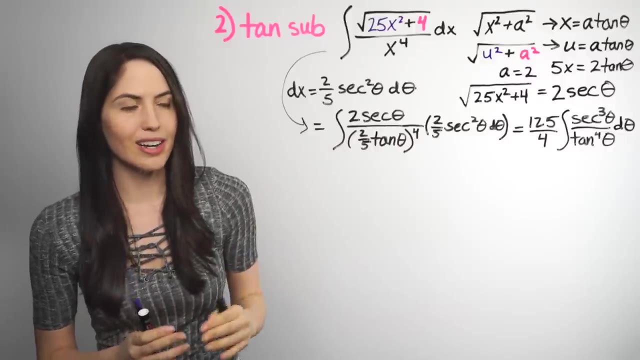 So how do you do that? You can try u-sub, you can try a table rule. They won't work. So what do you do? Anytime you have secants and tangents with powers divided or multiplied, or sines and cosines with powers divided or multiplied, it's a really good idea to try. 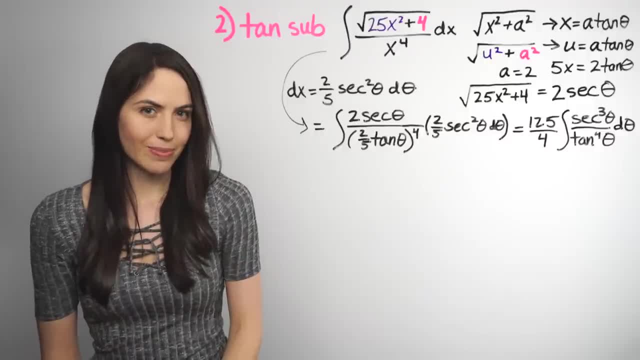 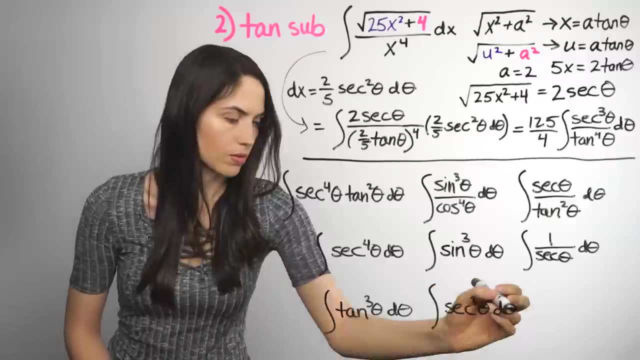 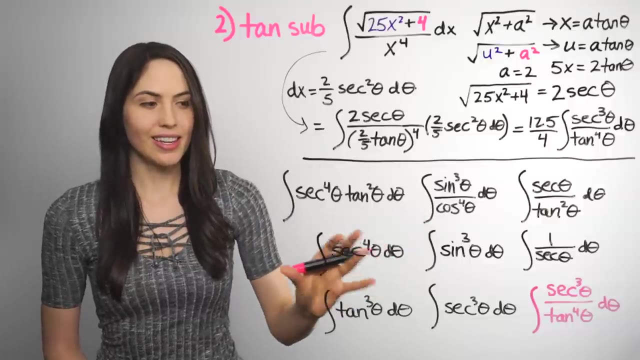 something called trig integral rules. Okay, let me help you out, All right. So if you're doing trig substitution and you wind up with an integral that looks like one of these, it is a really good idea to check trig integral rules, especially like: 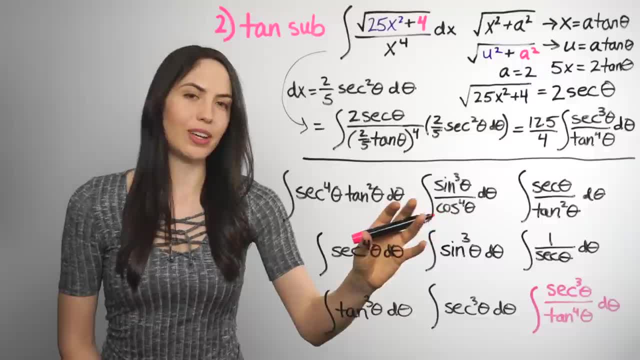 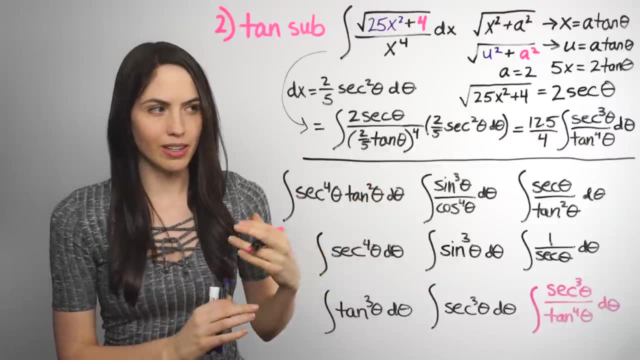 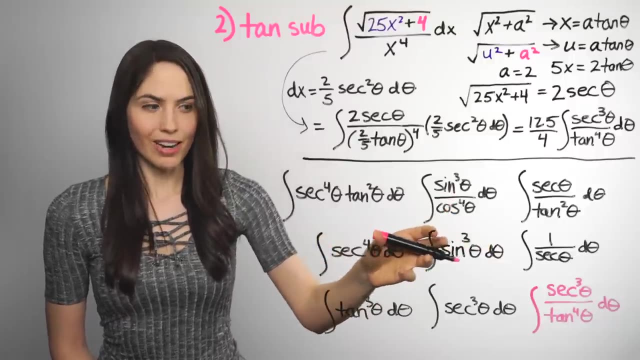 these here, And what those rules will tell you is generally to save one trig function and then convert the rest of it using Pythagorean identities. So, like for instance for this one, it'll tell you to keep one sine function and then take the sine squared that's left and convert that using Pythagorean. 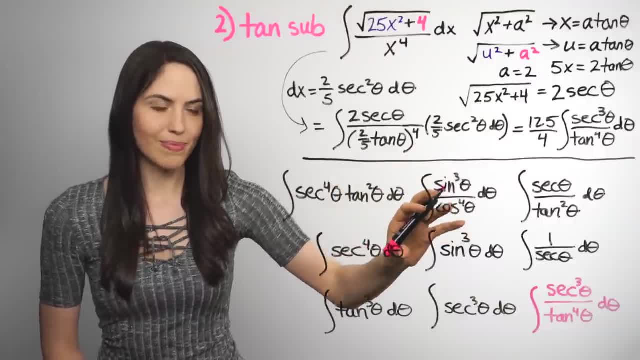 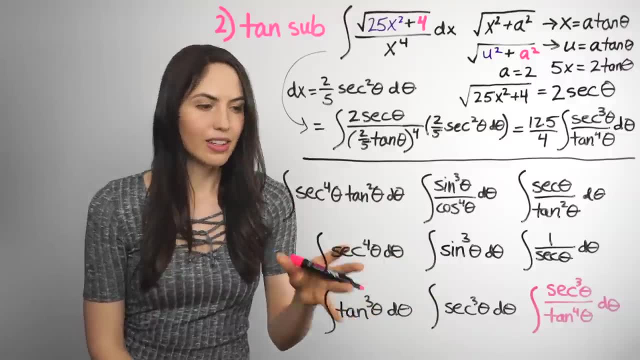 identity. Replace that with 1 minus cosine squared, Expand that and integrate and it will all work out. That's the idea for that type. So a lot of these fit that. I'm showing this to you because it's there's a really good chance that you'll run. 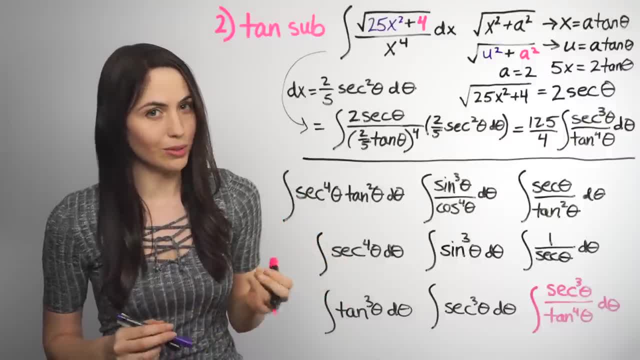 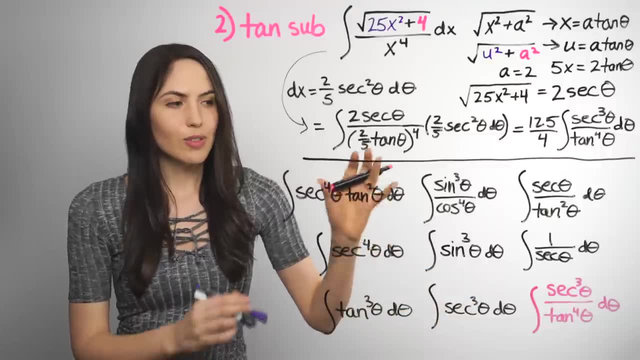 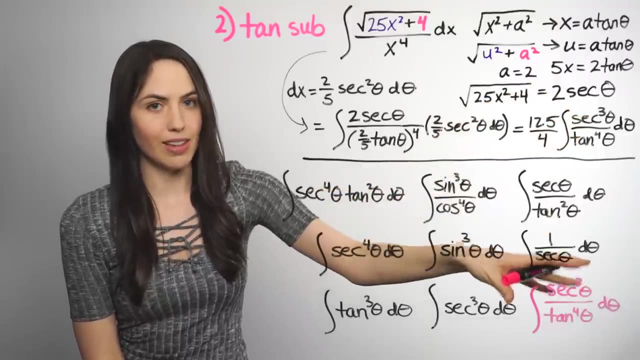 into one of these, especially if you've just learned about trig integral rules- And sometimes there's odd ones. like you end up having to use integration by parts for this one. If specific trig integral rules don't work, you could end up just needing to plain replace everything with sines and cosines and see what. 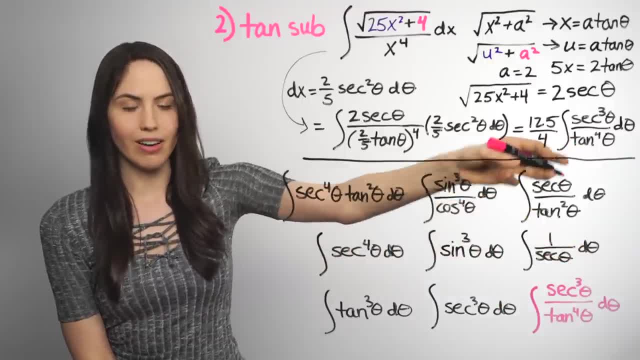 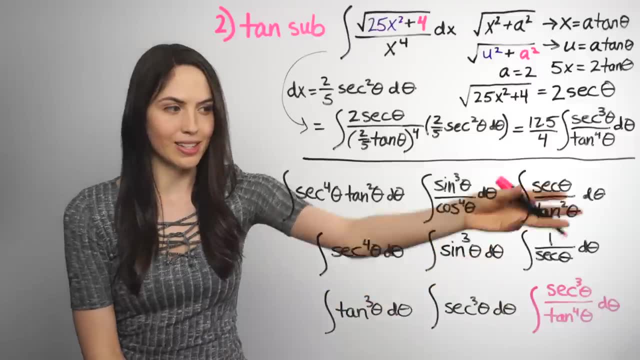 happens, Like here, like in general, if you have an odd secant power and an even tangent power like here or here, replace everything with sines and cosines, Here replace with cosines And then simplify it and hopefully you'll be able to use. 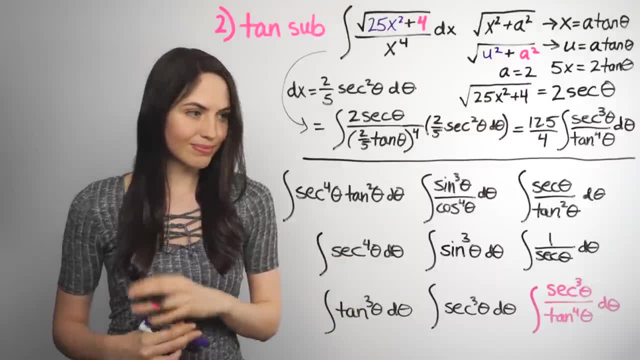 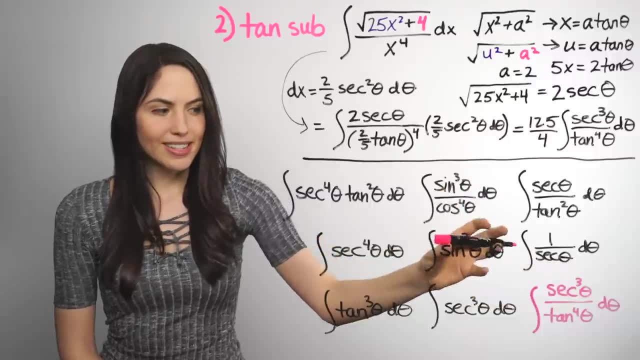 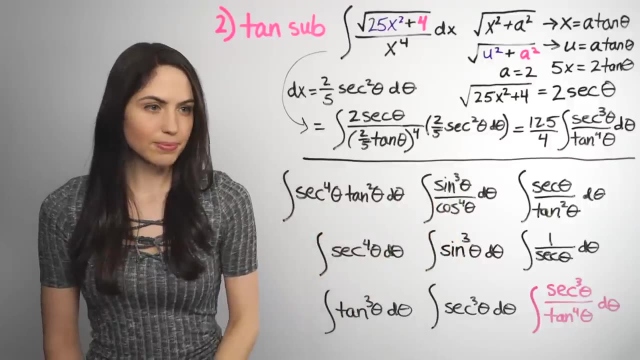 power rule or u sub or a table integral rule, And see if it works out. This is the one that we need here. that'll help us. So let's replace it all with sines and cosines that it's equal to and simplify it, and see how it turns out. 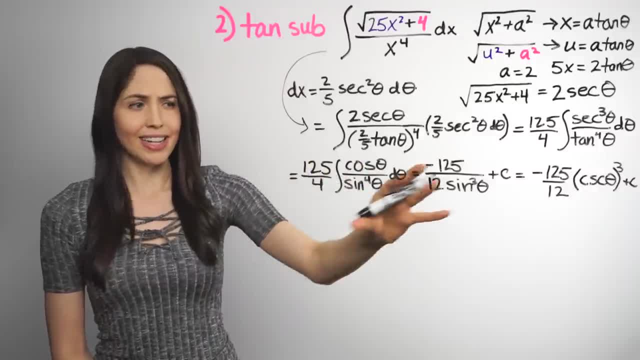 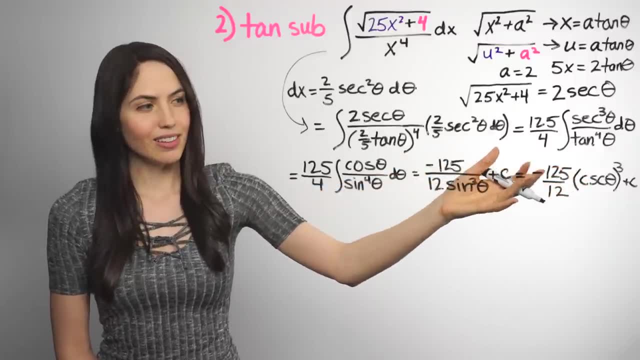 Alright, so replace everything with sines and cosines, clean it up, use the power rule to integrate and we get this answer which looks legit and all, but it has thetas in it And we need everything to be back in terms of x's to. 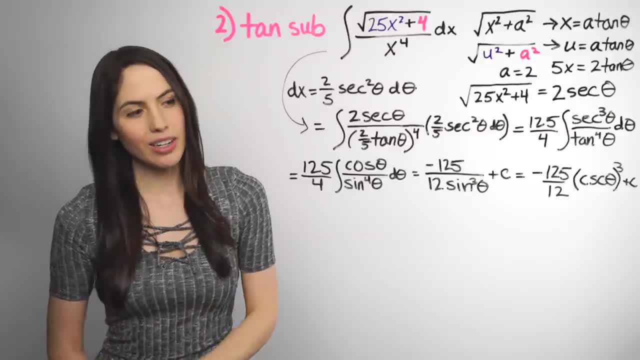 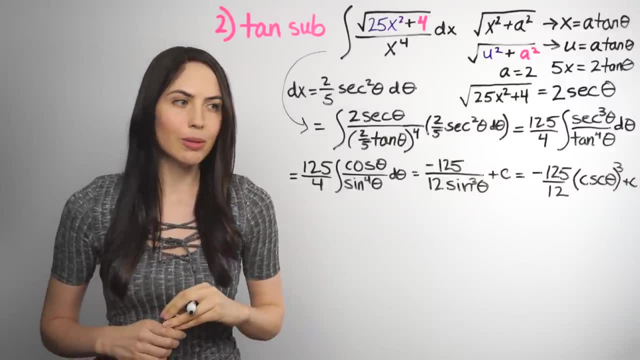 convert back to x's. So we have to do the side trig work. Don't be scared of the trig. Don't be scared of the side trig nonsense that we have to do at the end of these problems. I'm sure you've done much harder things at this point, So you've. 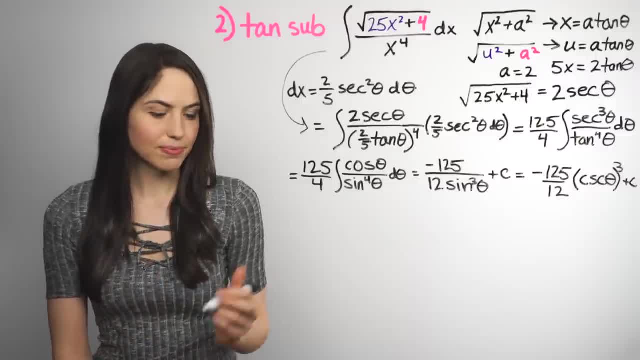 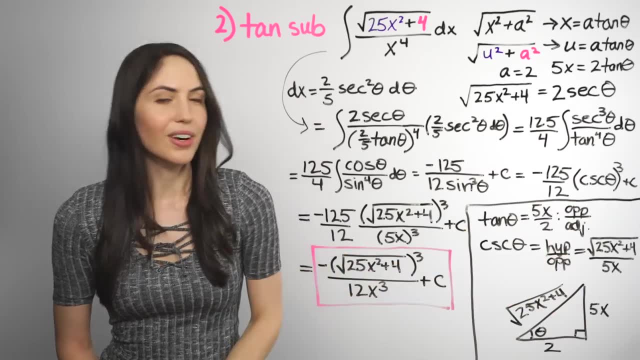 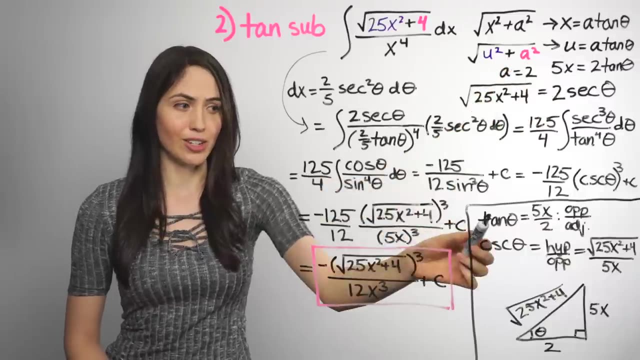 got this, Don't worry, And we're almost done. Okay, so the substitution that we have is the tangent one, And we know that tangent is 5x over 2.. Tangent is 5x over 2 here, And since tangent is the opposite side, 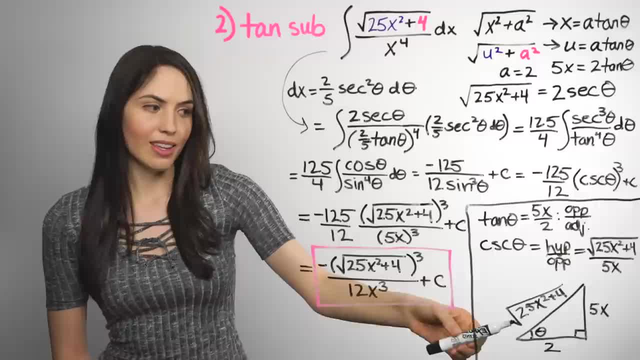 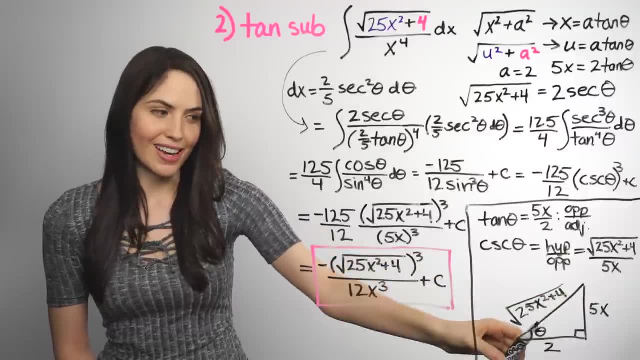 over adjacent side. we can label a right triangle with the opposite value over the adjacent value of 5x and 2.. And on the right triangle, since we have two sides, then can easily get the third side with the Pythagorean theorem. This should: 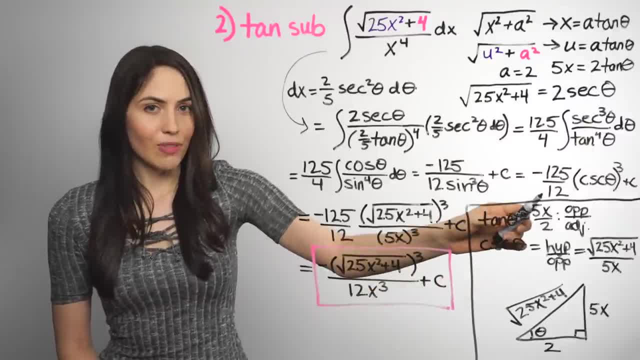 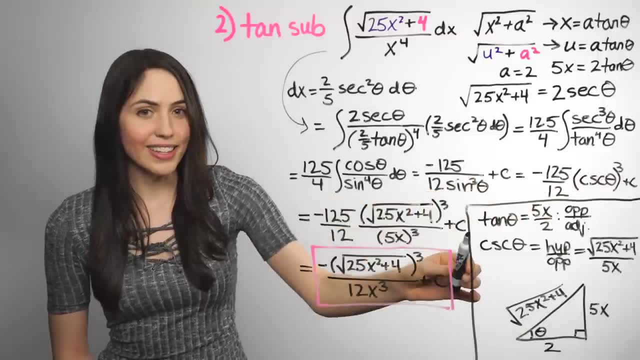 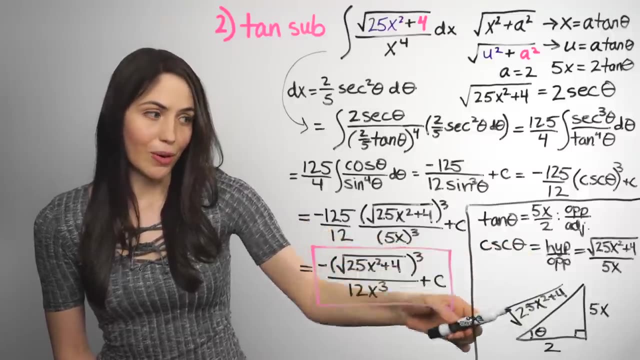 look very familiar to you. Subtitles by the Amaraorg community information that we used. but what we really need now in the end, is cosecant information, And since cosecant is hypotenuse over opposite, that will be equal to the hypotenuse value over the opposite value. So it's this that root. 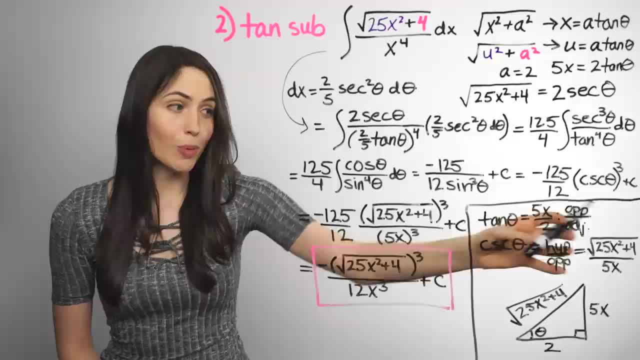 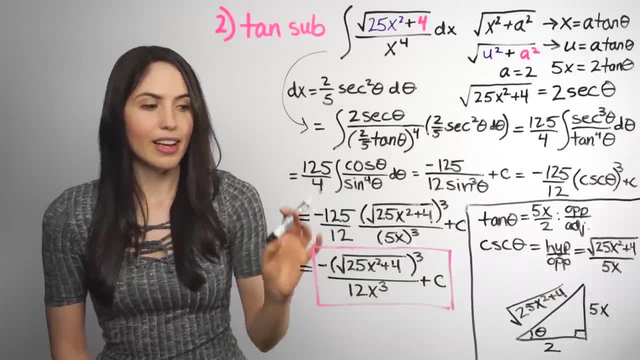 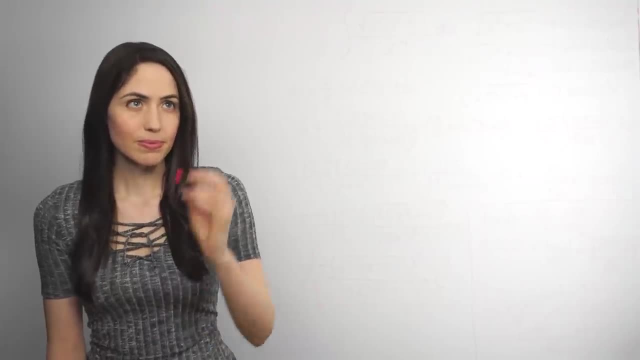 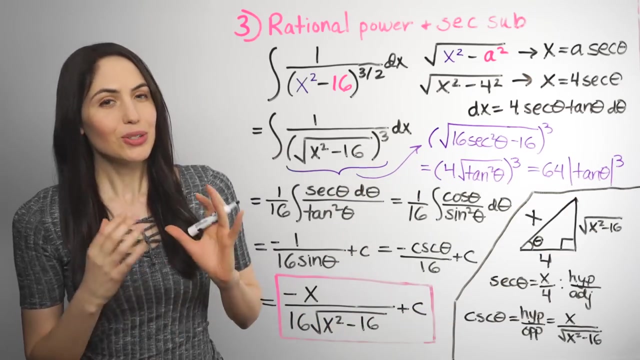 over 5x, which is kind of a mess. but that is what we will now put in place of cosecant theta, so that it's all in terms of x: Clean it up, and that's the answer for integral. So that is tangent substitution. Alright, don't be thrown off. 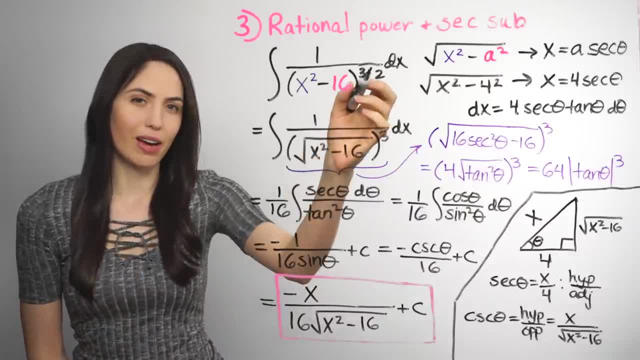 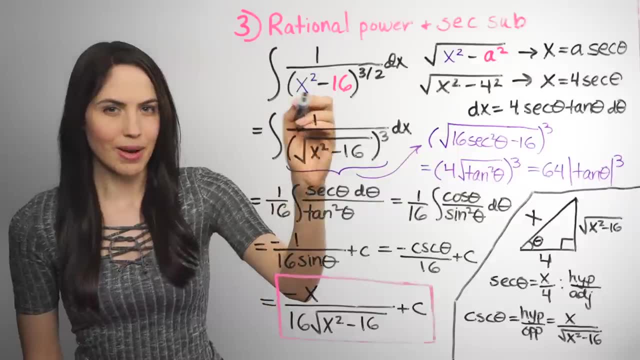 by weirder, different looking forms, like if you have a rational power, a fraction power, like 3 halves. But first of all, notice in this one this x squared minus a number, x squared minus 16.. This might look similar to the very first. 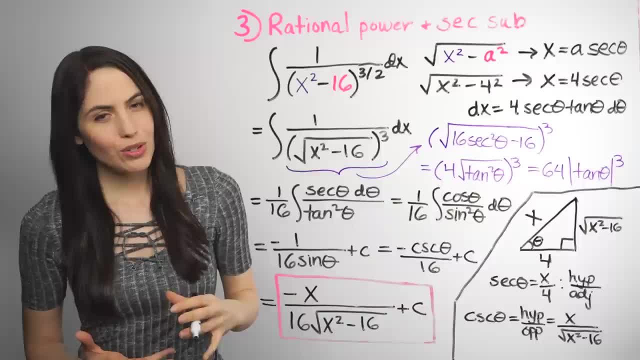 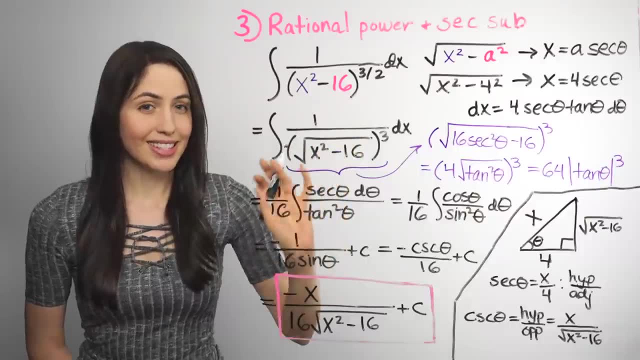 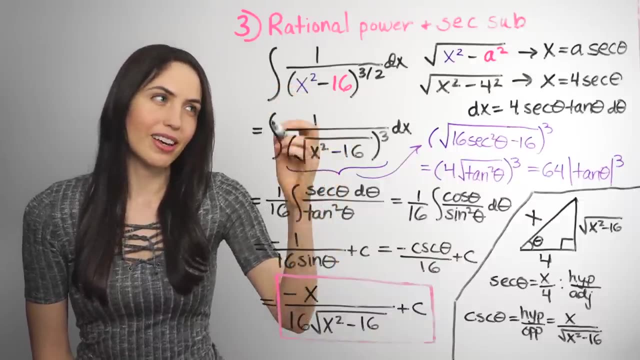 one we did, but that one was a sine substitution, and that was for when we have the form of a number minus x squared. This is the opposite, the reverse: When you have x squared minus a number, it's going to be a secant substitution. 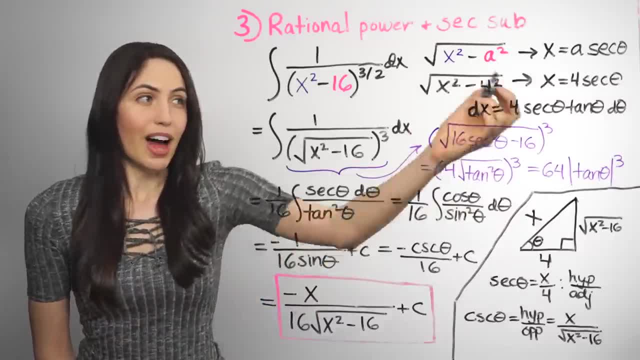 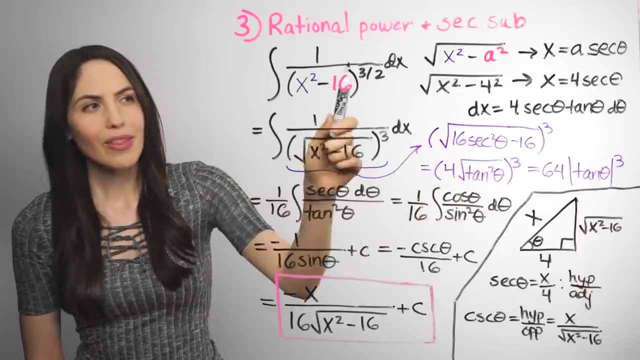 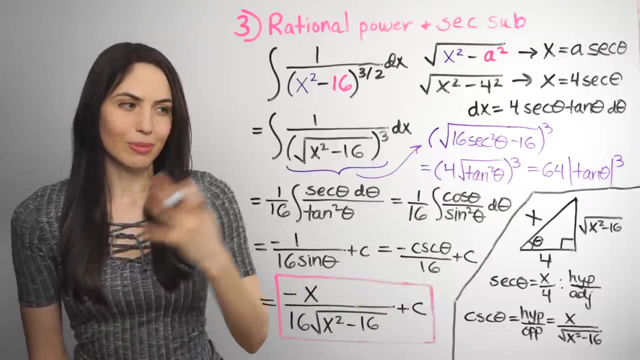 the last kind of trig substitution And we will have a equals 4, our substitution will be x equals 4 secant theta. But what about this 3 halves fractional power? Can you even do trig substitution when you have something like that? Well, you can probably tell already that the answer is yes. 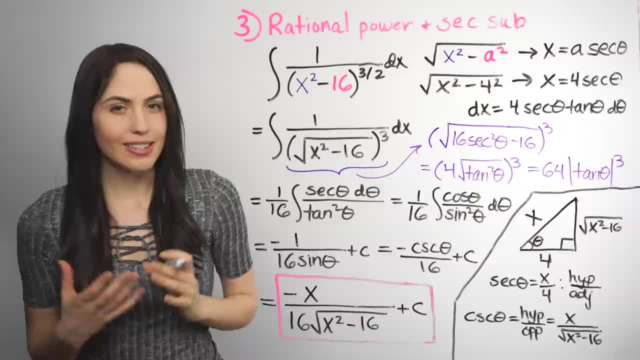 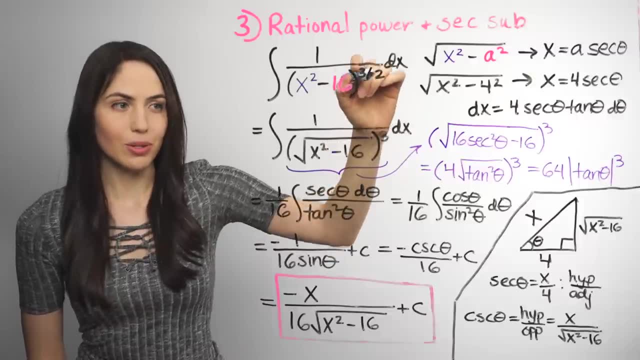 I've already written out the work for it, But the trick to see it is to rewrite it as a root raised to a power, Like in the power, the bottom 2 means a second root, square root, and the top 3 means raised to the third power. So write it like that so that you can really 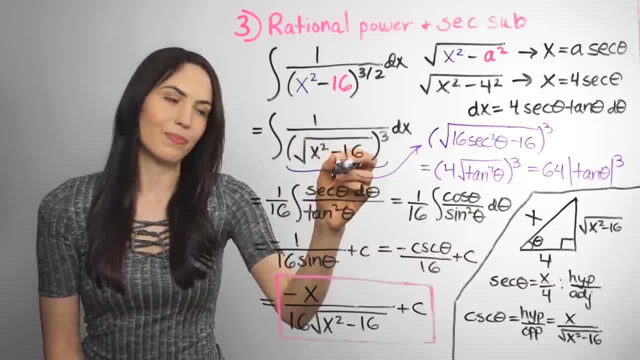 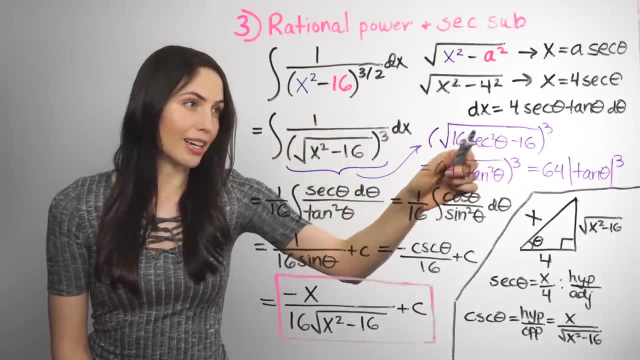 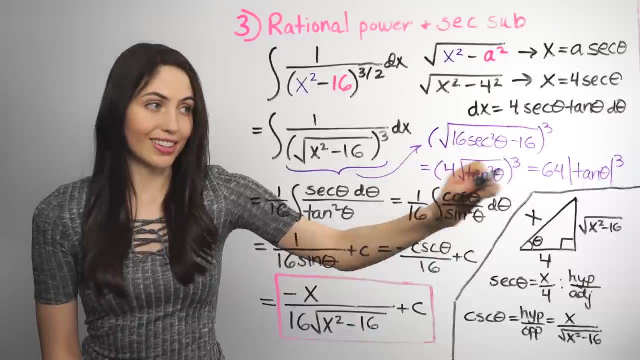 see what it is, It will be easier to do the trig substitution. I took the whole denominator and substituted into that. If you plug it in, simplify, use a Pythagorean identity that secant squared minus 1 is tangent squared, You'll get this. 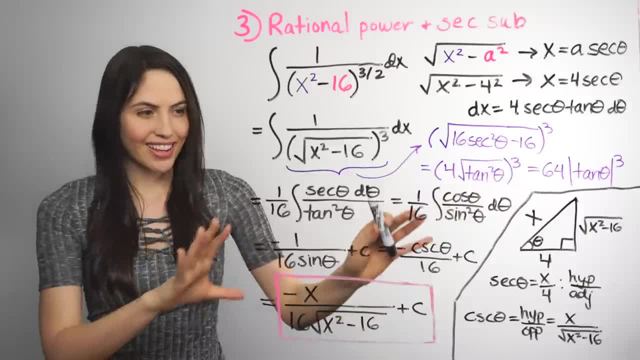 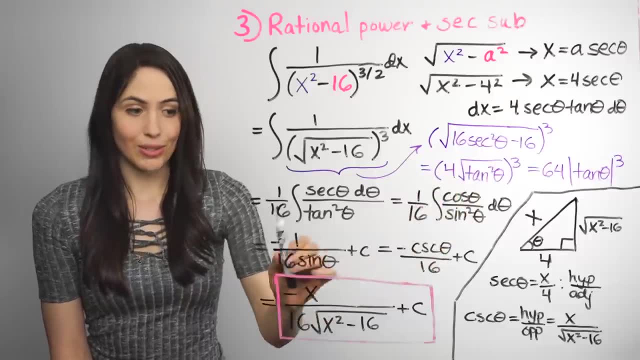 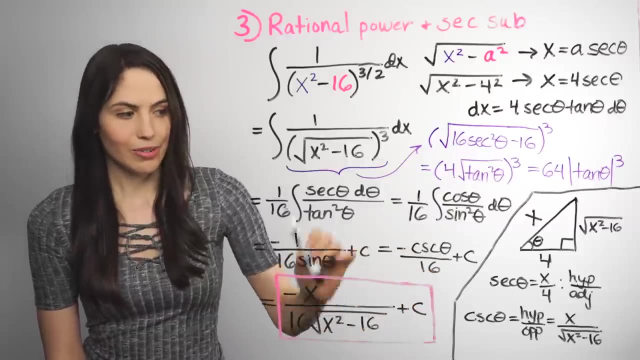 You can drop the absolute value bars, plug everything in. simplify ends up being one where you replace with cosines and sines. Then you can do straight up power rule and you get this answer After you back substitute in to get all in terms of x's with your right triangle trigonometry. 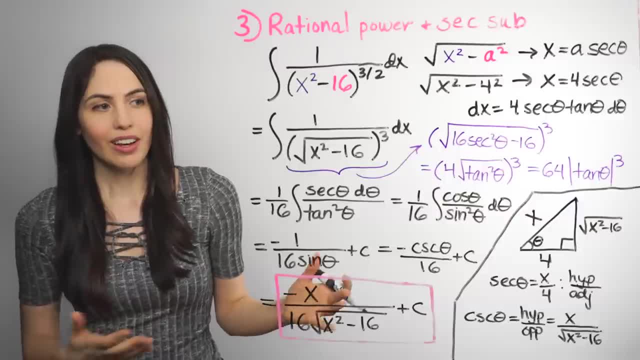 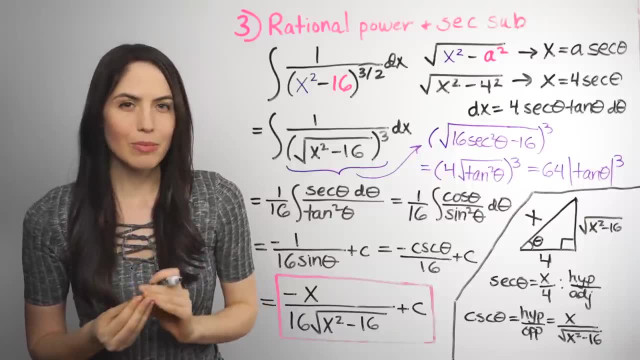 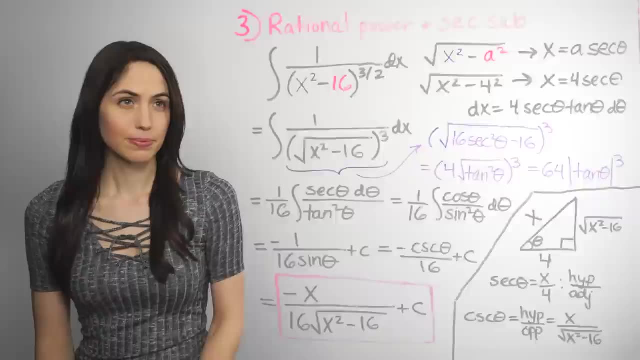 that's the answer. So this is how you do secant substitution and also how you handle a rational power like that. Let's fiddle with the forms a little bit more. Let me show you some slightly even weirder kinds where you can still use trig substitution. 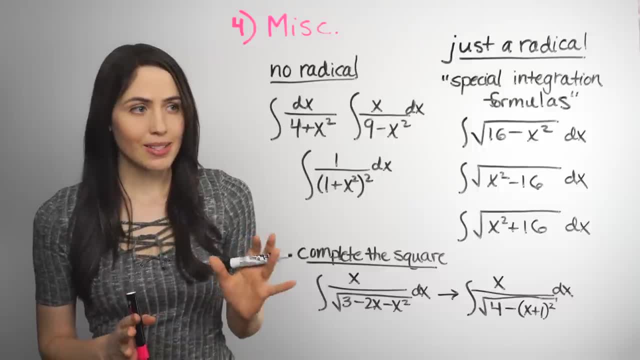 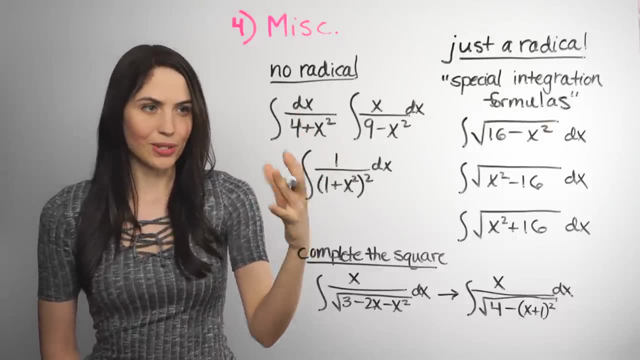 Finally, here's some kinds that might not look like. you can use trig sub, but you can Like if there's no radical in the integral at all turns out. you can use trig sub if it still looks like one of these forms, Even though it might not be the fastest way, like 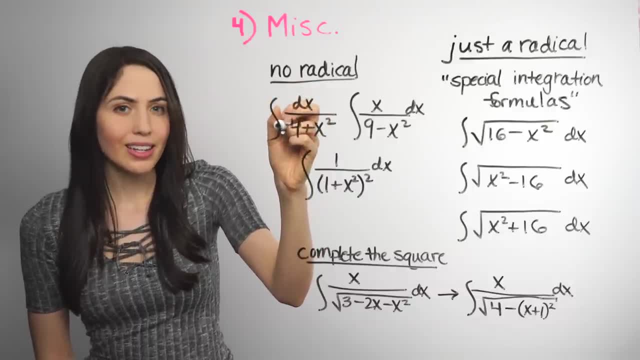 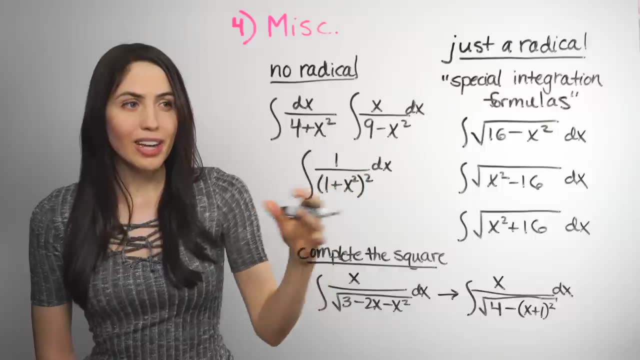 this one. it would be a lot faster to use the arctan integral rule or the inverse tangent integral rule. Here. it would be a lot faster to use the u substitution. But you can use trig sub if you want to. You can also use trig sub as an integral If you're looking for a. 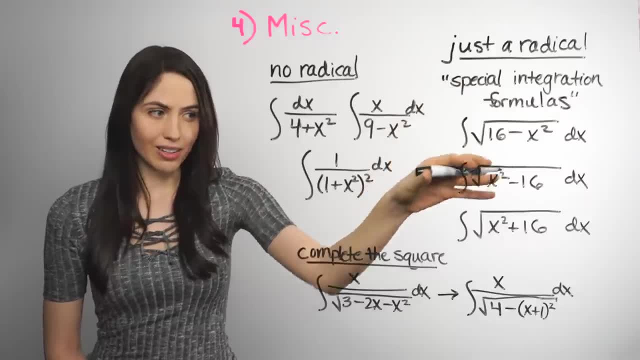 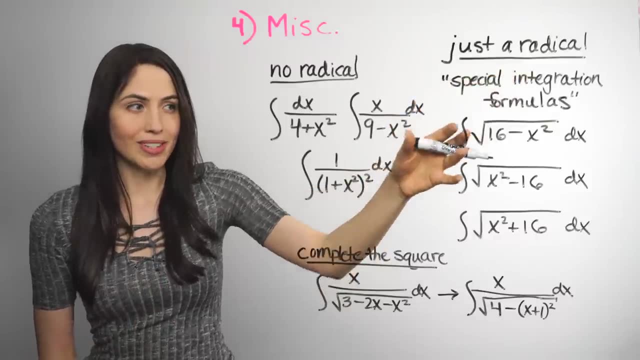 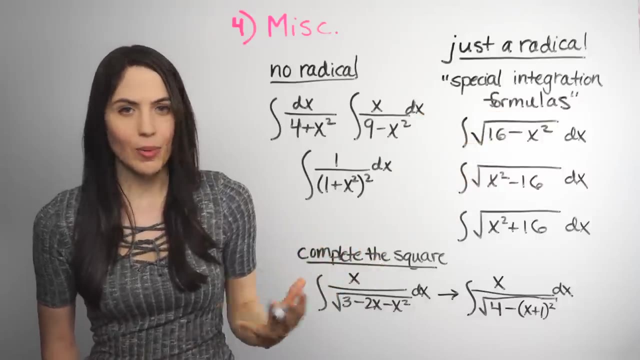 or if you have to Here, if you have just a radical in the integral you can do trig substitution. If you're really lucky you might get special integration formulas that tell you right away with these specific kinds equal. If you're not so lucky you won't get those. But either way, 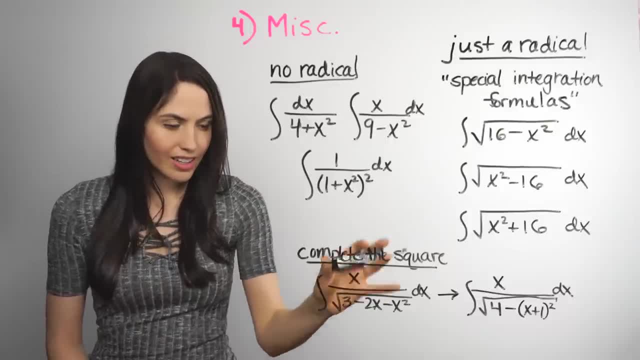 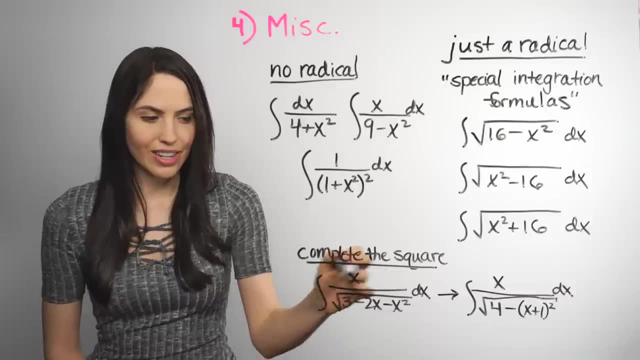 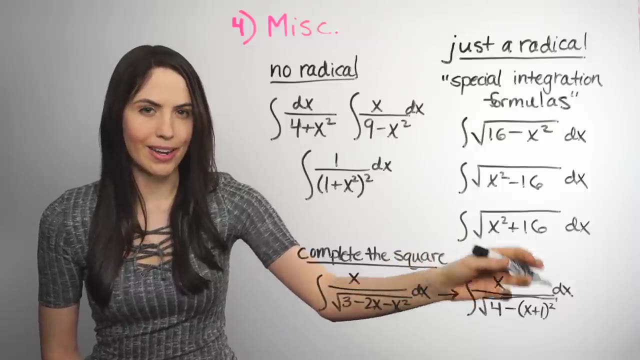 you can do trig sub And then finally, something like this does not right away look like a trig sub form that we saw, but you can use a little algebra completing the square to make it look like that and do some magic to get it into this form of a number minus an x squared term And